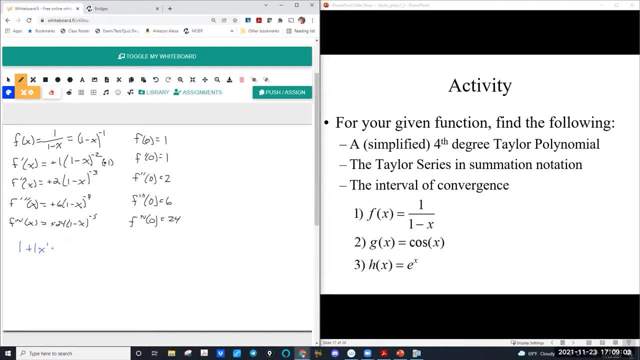 If it was centered someplace else, we would put x minus in parentheses. Plus, our next term is going to be two over two factorial x squared. Our next term is going to be two over two factorial x squared. Our next term is going to be two over two factorial x squared. 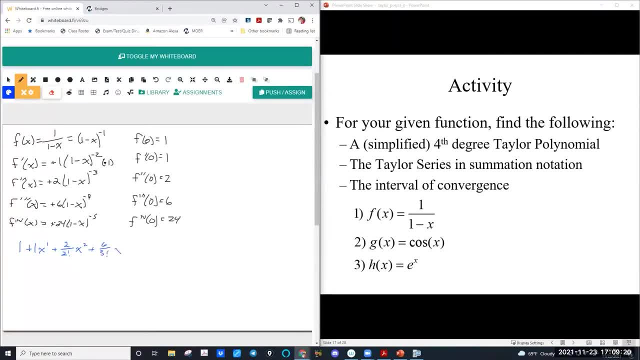 Our next term is going to be six over three- factorial x, cubed. And then, because we're asked for a fourth degree, we need something raised to the fourth power. so we need the next term, So 24 over four. factorial x to the fourth. 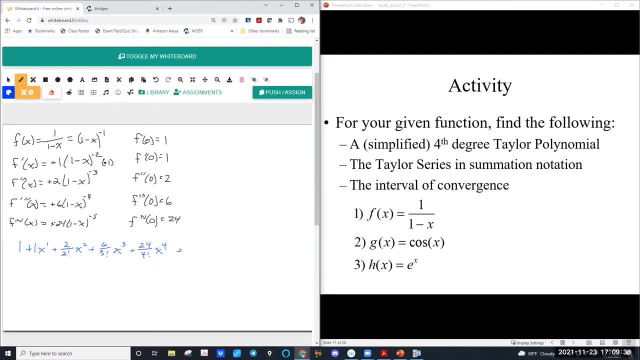 Now we're going to simplify this as much as possible to see what this looks like. So we have one plus x And then two over two factorial, That's just one Those cancel. So plus x, squared Three over three factorial. 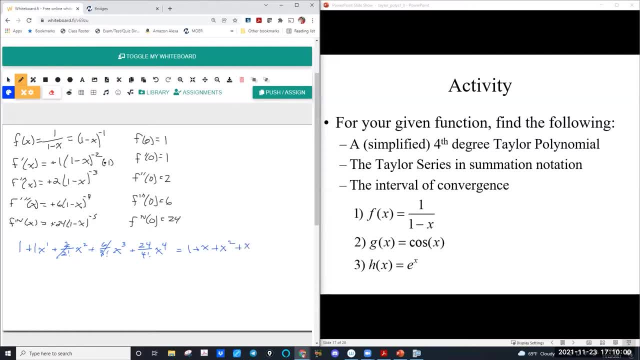 Well, those cancel Three, factorial is six, so it's just x cubed, And we see this pattern emerge really quickly. All right, So this is the fourth degree Taylor polynomial And if we want to maybe give that a name, piece of four of x. 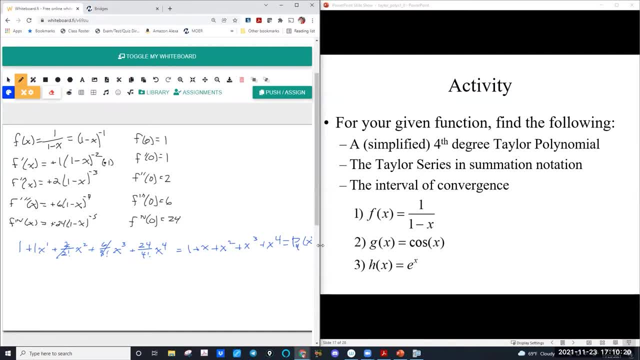 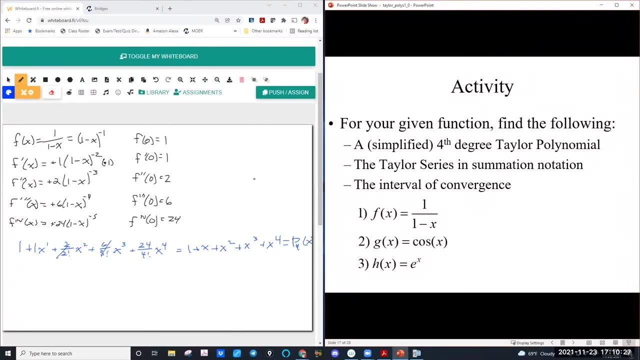 That's our fourth degree Taylor polynomial for the given function centered about zero. Again, this is going to start off as a little bit of review, But if you have questions, let me know. These terms would just keep going like this infinitely. So to write this thing in summation notation: 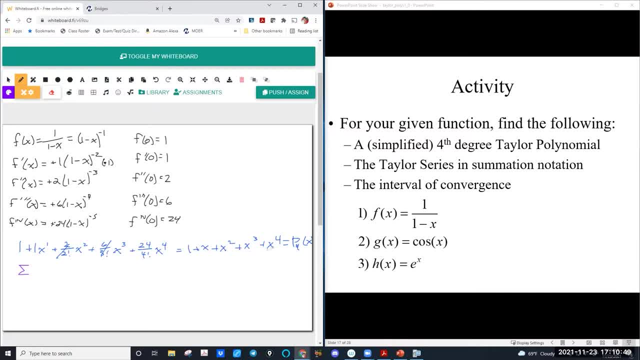 We have this, We have the sum of this is actually not a bad one, right? It's just basically going to be x to the n If we start at zero, because that'll make x to the zero, which is one Started at zero up to infinity. 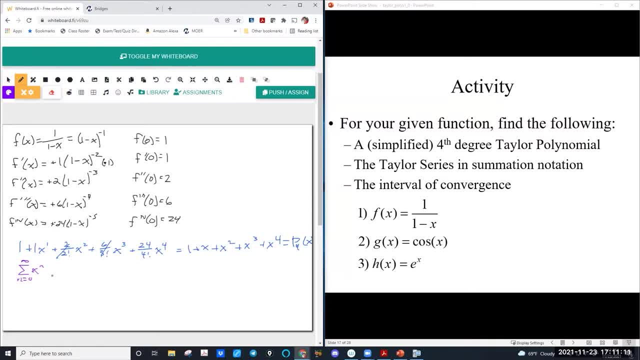 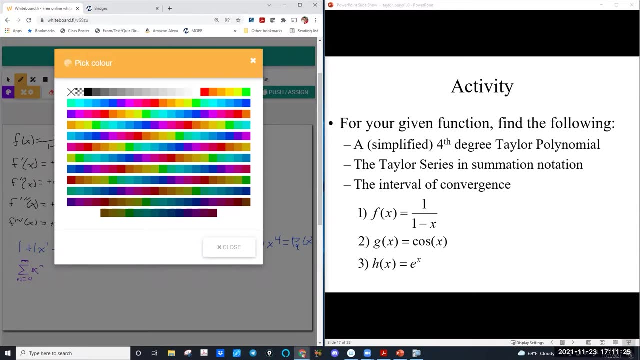 So that's going to be the Taylor series of one over one minus x. Now we want it in this closed form so we can do the Interval of convergence. As we saw last time, the interval of convergence basically means we want to apply our ratio test. 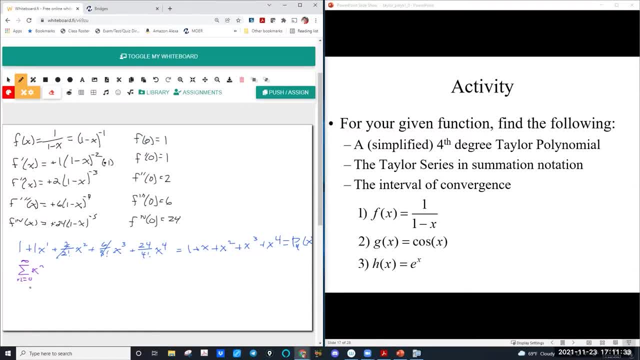 So We want to apply our ratio test here. So we have the limit As n goes to infinity. a very easy one to set up: X to the n plus one over one times the reciprocal. n plus one over one times the reciprocal. x to the n plus one over one times the reciprocal. x to the n plus one over one times the reciprocal. n plus one over one times the reciprocal n plus one over one times the reciprocal. I said it but didn't write it. 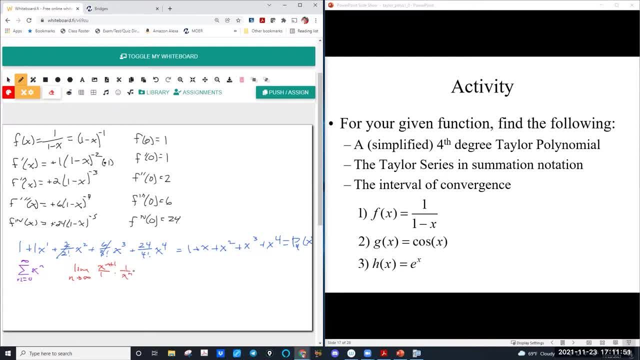 Times one over x to the n, The absolute value- Now we know from our canceling It becomes limit as N goes to infinity- of basically just the absolute value of x, Which is actually equal to the absolute value of x Because there's no n. 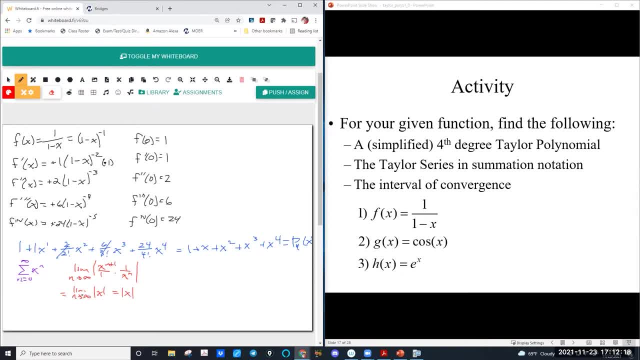 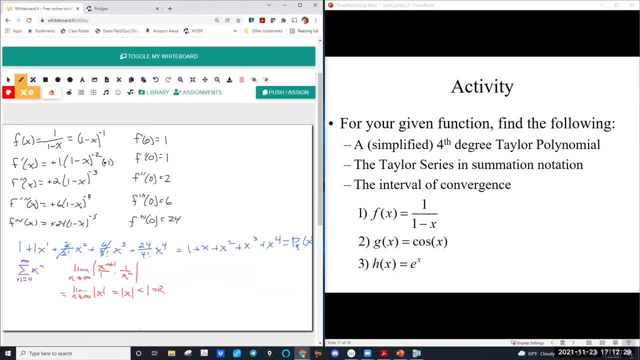 So, right off the bat, our radius of convergence is one. Now to do the interval, we have to check the endpoints. This is what we were working on last time. So we know that x is in between one and negative one. So those are two endpoints. 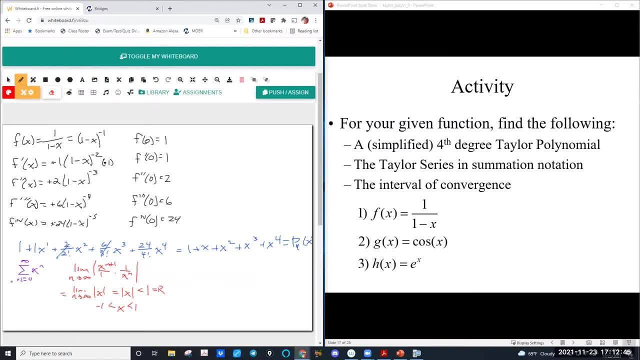 So So. so if we check our endpoints, so first off we check one, well then our series becomes one to the n, or just the summation of one which goes to infinity. so this diverges, because this sequence does not go to zero. we could call it our divergence test. so by our divergence test, 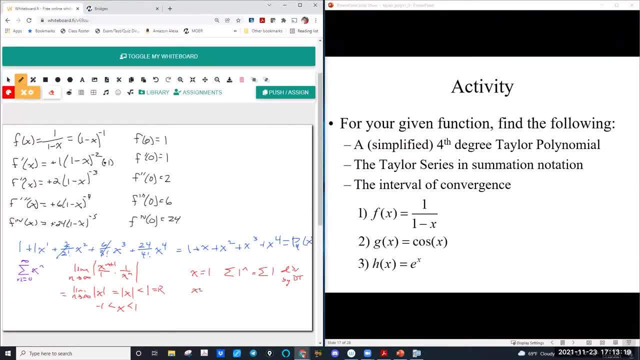 similarly, even if x is negative one, we have negative one to the n that literally just flips back and forth between one and zero. so that actually does not have a sum either. and we could use the same argument: that sequence does not go to zero. it's also divergent by the divergence test, so we don't want to include either endpoint. 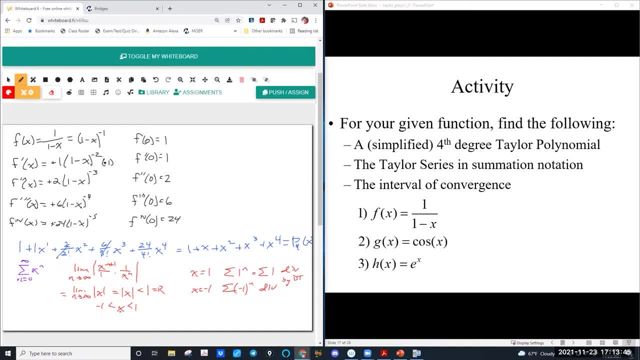 so our interval of convergence is negative one to one. we can put this in interval notation if we want, but we don't want to include negative one or one. now. there's a couple reasons that i specifically picked this series number one. let's- uh, let's write this out so we can kind of see: 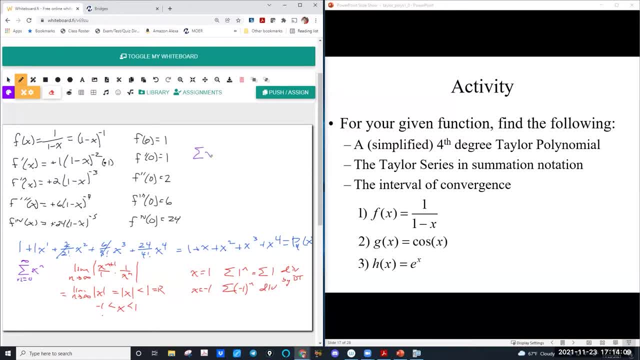 what's going on? the series of x to the n, n equals zero. to infinity is equal to one over one minus x. well, we've encountered this before, when x was our common ratio. so, if we think, if we think of this, as this is an exponential function, so this is basically geometric. remember the sum of an infinite geometric series. 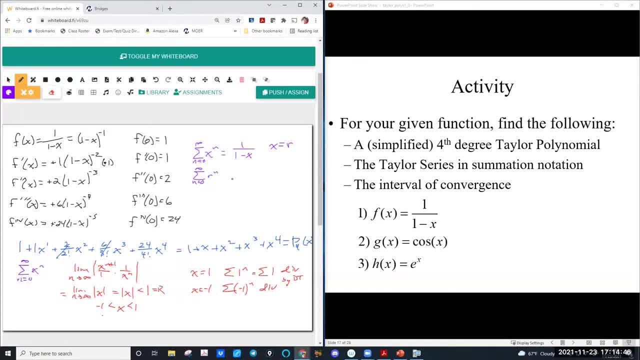 with a common ratio of r is equal to the first term, over one minus the common ratio. if that common ratio is let, the absolute value of it is less than one. again, exactly what we found here. we actually did this in the reverse, so back in section 8.2. 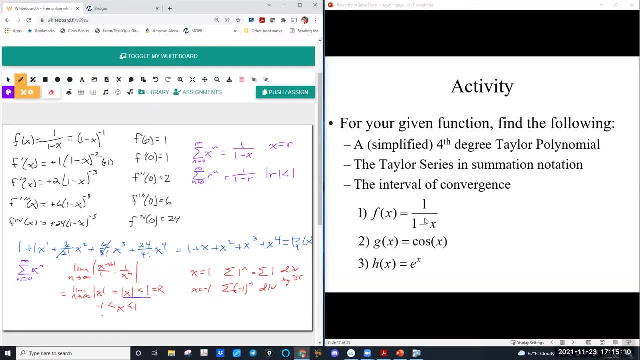 of ourды in the lesson. this formula was derived for the sum of an infinite geometric series. now what we're doing is we're taking the formula of the infinite geometric series using taylor series, finding its taylor series to show that it is the sum of an infinite geometric. 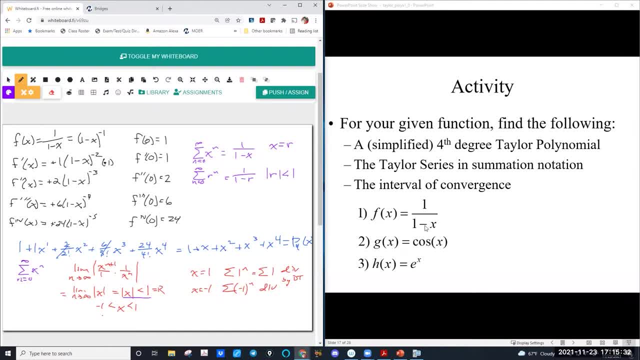 so part of the reason i chose this one is i love making that connection because it's something we've seen before. we're just now doing it in the reverse. the other reason why i'm doing it in reverse is actually one of the urgent reasons to remember. this says: wow, this trees, this tree here, just kind of come out all of the way out of this wall right here, sqm notet. so is that kind of ways that we can? 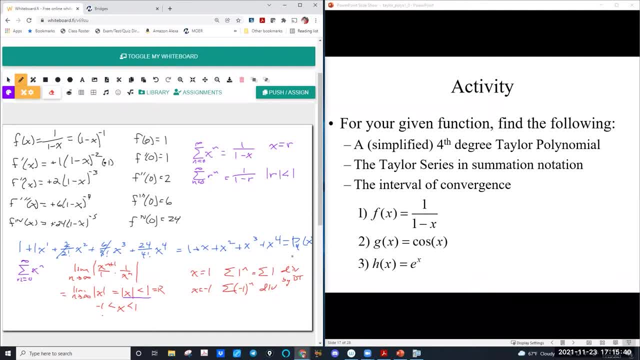 the other reason why i'm doing it in reverse is because we all we miss czyli that if you are going to do such a solution to that distribution and say: well, we're gonna, Mister Polangenko. So another reason that I like that we're using this one is we're going to modify this and see how we can use a known Taylor series to find more complicated Taylor series. 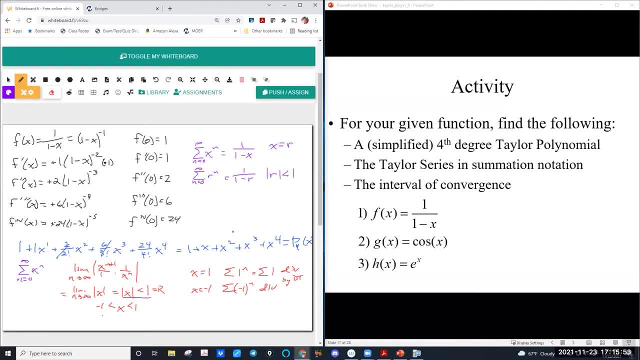 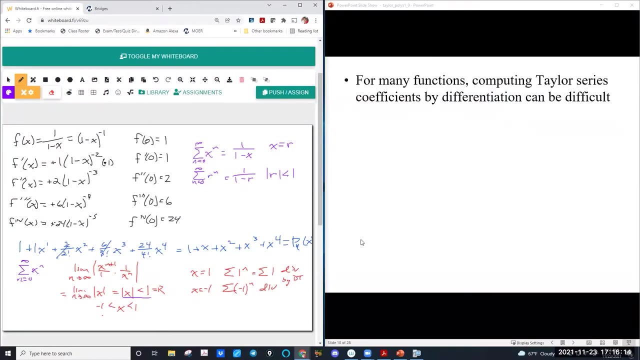 But before we go into that, Any questions about this first one? Okay, we need that foundation to go and do some of the other stuff we're going to do Now. let's talk about using a Taylor's unknown Taylor series to find a more complicated Taylor series. 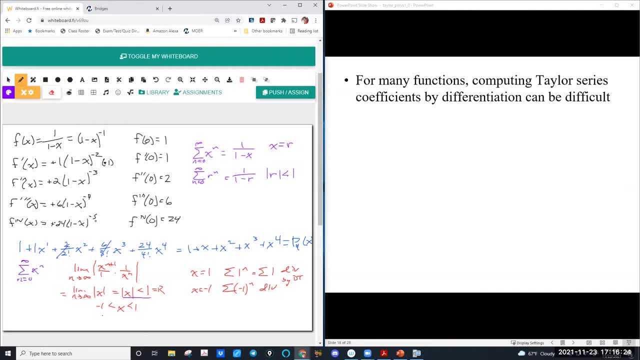 So, as you just saw, to find the Taylor series we had to take a bunch of derivatives. this one wasn't that bad. it did involve chain rule, but really not a bad chain. But what if our function was something like a polynomial times, a trig function? 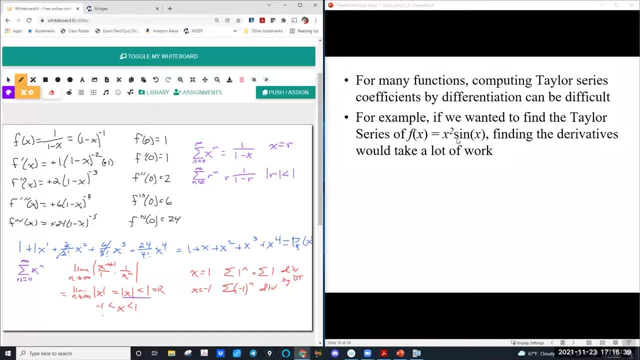 All right. first, derivative needs product rule. Well, these derivatives get increasingly more complex because of the need for chain rule. So if we wanted to find six or seven terms, this could be a lot of work, But we can use what we already know. 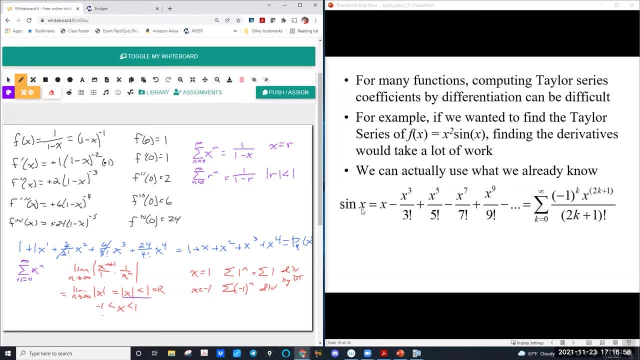 We know the Taylor series for sine of x, So the Taylor series for x squared times sine of x. we just multiply all the terms by an x squared. So what's happening here And I just want to make it real obvious and let me know if you have any questions about that. 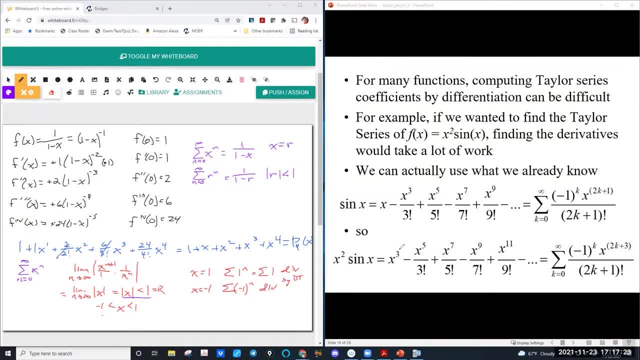 This. but what's happening? Notice all the terms. Now have an exponent that's exactly two higher. So what we did is we took this guy and we multiplied it by x, squared. Well, what did that do that? We increased all the exponents by two. So, in the closed form, 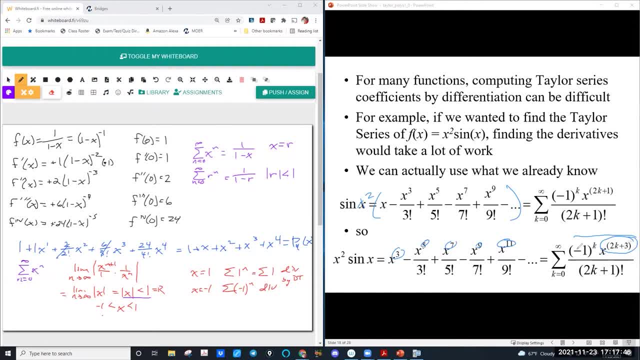 Our exponent is now exactly two higher. We did not have to take a single derivative of x squared times sine of x. Okay, this is what's called using a known Taylor series to find more complex and more complicated functions. So if we have the Taylor series for this guy, we will look at a more complicated version. 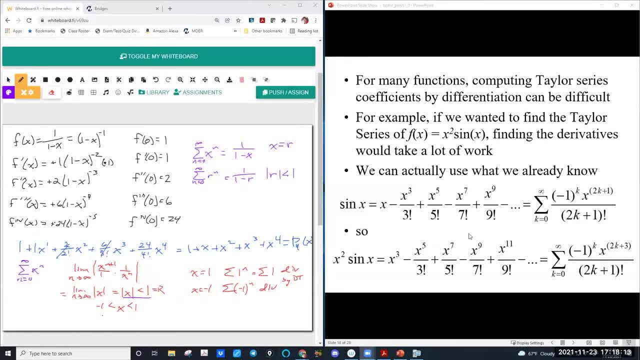 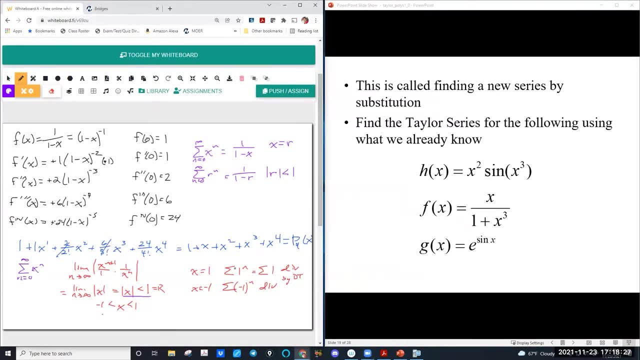 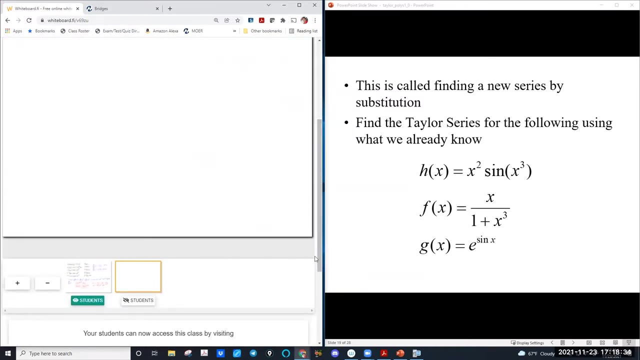 But before I go on any questions about about this idea, Okay, let's see how this plays out. So, let's see, I'm going to need to go to a new slide Right Right now. we know, Okay, so, what we learned in that first slide that we're going to bring up. 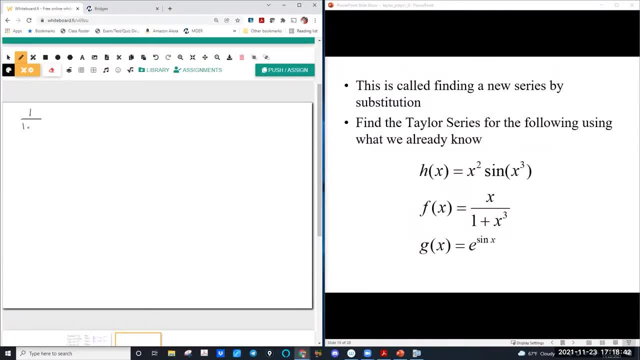 Here's what we already know. we know that one over one minus x is equal to the Taylor series from n equals zero to infinity of x to the right. that's what we saw last time and if we wanted to write that out, it's one plus x plus x squared plus that. 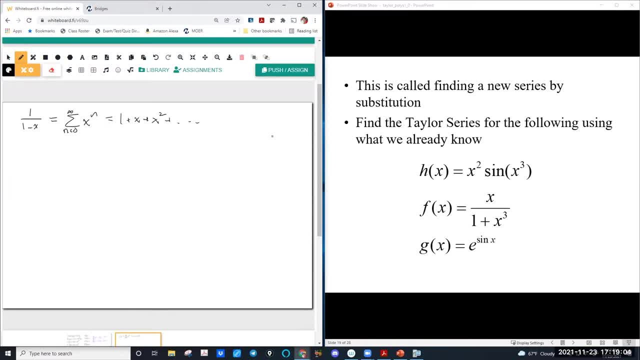 Now we're going to look at the middle one, because that's the one that's set up for the one. That's the one that's set up for the one we're working on Now. I showed you how it works for multiplication. I'm going to show you how it works with a composition. 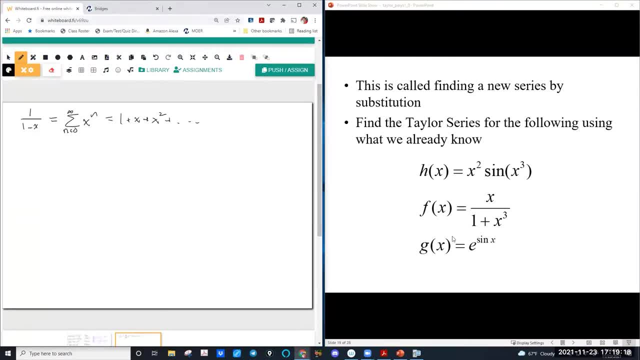 All right, So I'm going to do this in a couple of different steps and I'll use different colors to identify. the first thing we're going to do is we're going to take care of the one plus x cubed. How do we make this look like that? 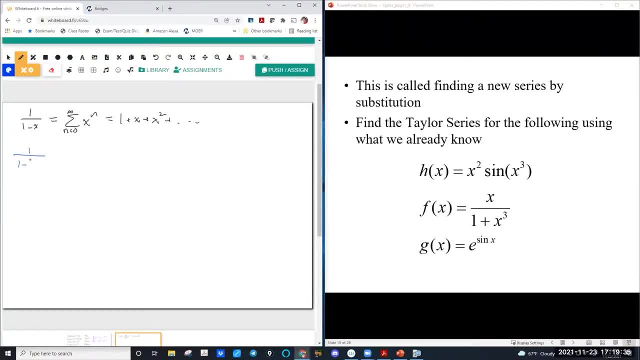 So one over one minus a negative x cubed, That's equal to one over one plus x cubed. The way it relates to the first one is we have a composition. All the x's are getting replaced with a negative x cubed. 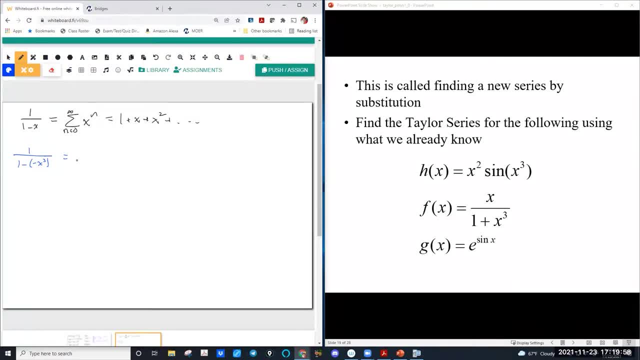 Let's, let's do it in this form first, and then we'll probably should have written these the other way. So one plus Negative x cubed, plus Negative x cubed, squared, plus Negative x cubed to the fourth. I think that's plenty of terms. 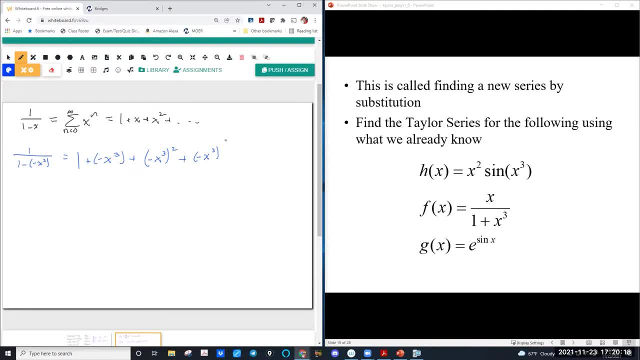 Excuse me to the first, second, third. I think that'll be enough terms for us to see. We need more. we can always put them in. And then we got to figure out, okay? well then, there's the summation, All right? well, n equals zero to infinity. 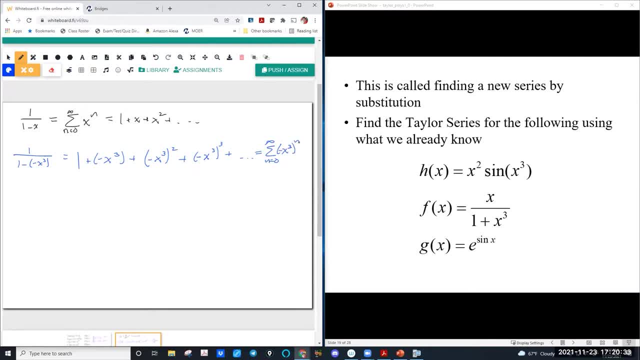 Of negative x Cubed to the n. All right, I want to simplify what's going on here because I want you to see something. So we have one Now. it's negative when the exponent is negative. So one minus X cubed. 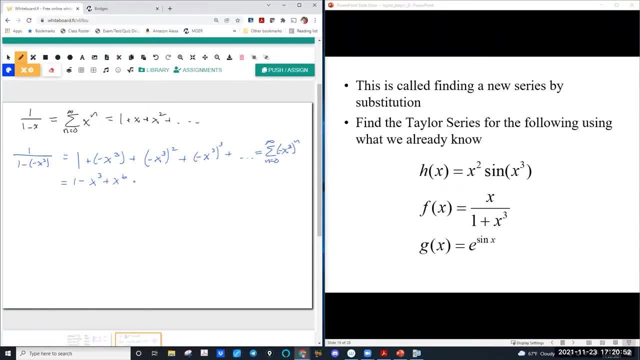 This one is going to be plus X to the six, Minus x to the ninth. You can probably start to see the pattern plus x to the 12. And so forth. All right, Now we want this Summation notation to match up. 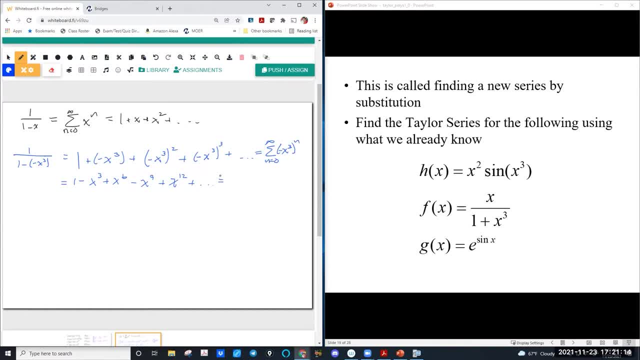 It's all in here, but we're going to make it look a little cleaner. Right off the bat We see that it's alternating, So I'm going to split off the alternating piece, the way we're used to seeing it: Negative one to the end. 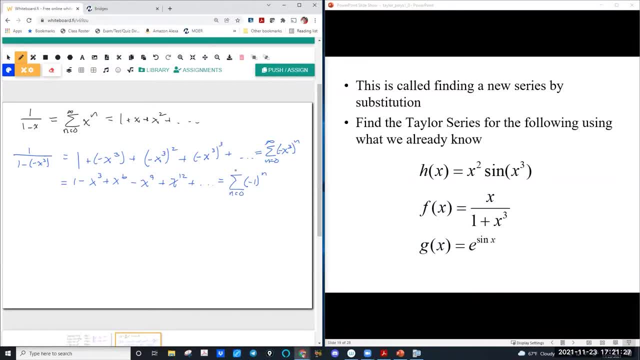 So I'm just taking that negative and raising it to the end And then X to the three to the end We'll be rewritten X to the three And we can see that. Okay, The alternating plus minus plus, minus, plus. Okay. 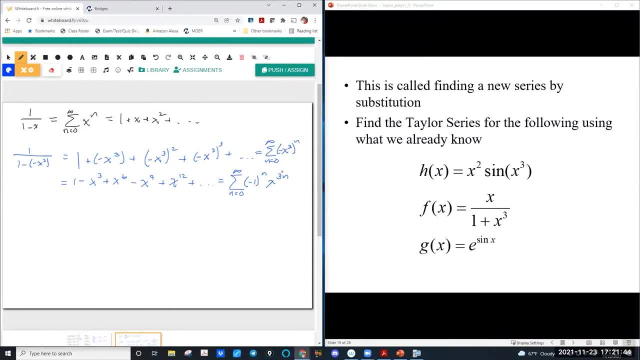 That works. And X to the three: N. When N is zero, we get one, When N is one, we get X cubed. When N is two, we get X to the six. So We have now found the Taylor expansion for 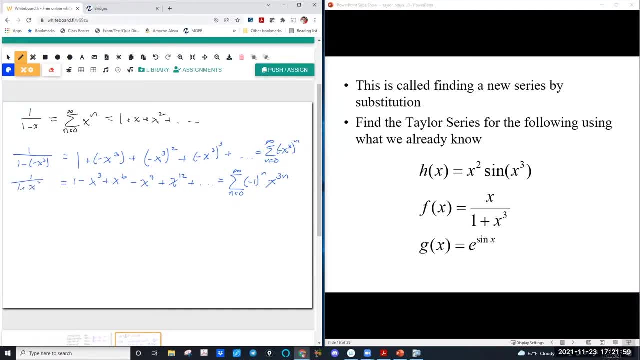 That's right. This way We have now found the Taylor expansion for One over one plus One over one plus Excuse. So We've taken care of how we make the denominator Do that. We do it via composition. 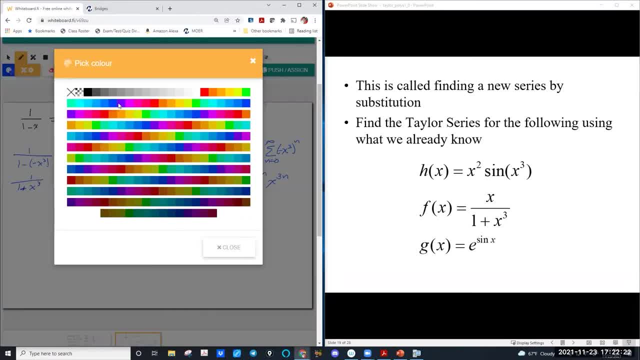 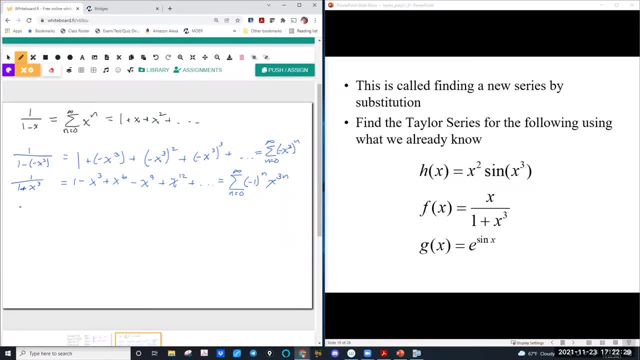 Questions at this point, All right. Well, we were asked to find X over one plus X cube. Well, basically, we're thinking of it as X Times one over One plus X cubed, So everything's getting multiplied by X. 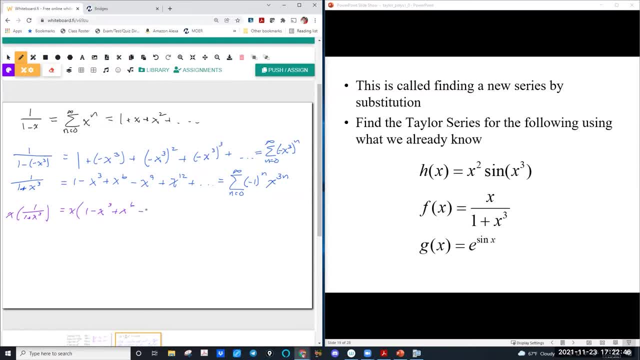 So minus, execute, plus X to the six, Minus X to the ninth, plus X to the 12th, It's dot dot dot. And then this is getting multiplied by an X, So Negative one to the N, X to the three N, and then times that X. 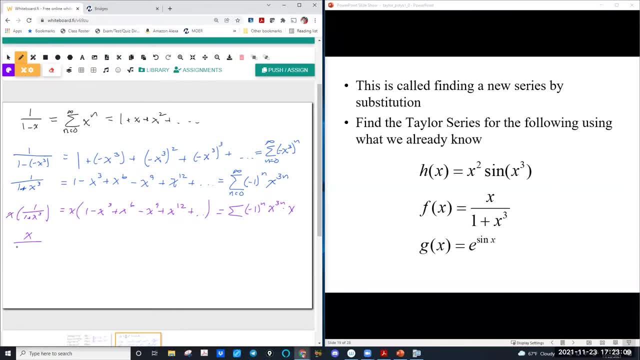 So We wanted the Taylor's expansion for X Over one plus X cube. We're going to just basically distribute that X to all these terms, which really just raises the exponent by one. So X Minus X to the fourth, Plus X to the seventh. 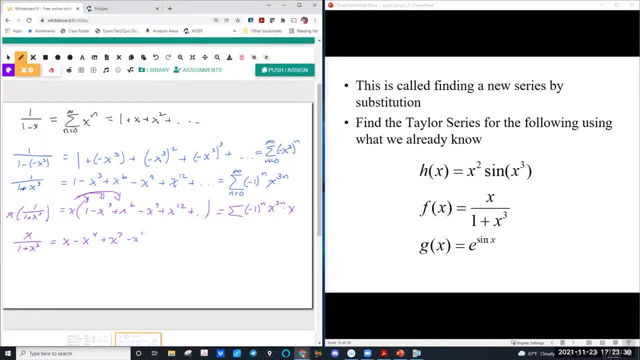 Minus X to the 10th, Plus X to the 13th, So on and so forth. And then for our summation We have negative one to the end. We can combine those because they have the same base. That would be X to the three N plus one up in the exponent. 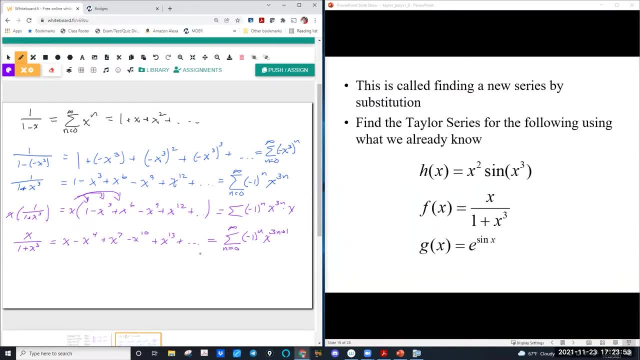 Still going to start at zero, still going to go up to infinity. And what we've done is we've found the Taylor expansion For this function Without having to use quotient rule and product rule and chain rule to take the derivatives. That is what's known as using known Taylor series. 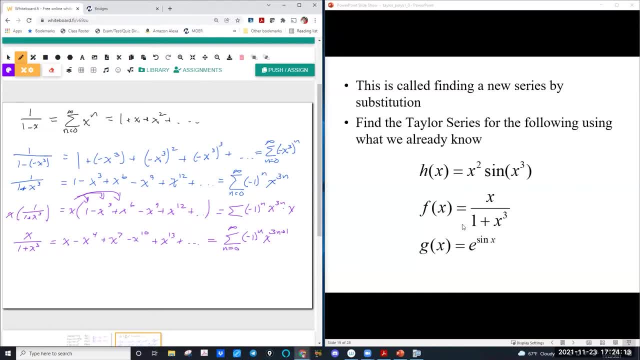 To find other Taylor series Saves a lot of time on some of these more complex functions. You'll get to practice a couple of these in the homework, Where you're taking a known Taylor series and using it To To derive another one. 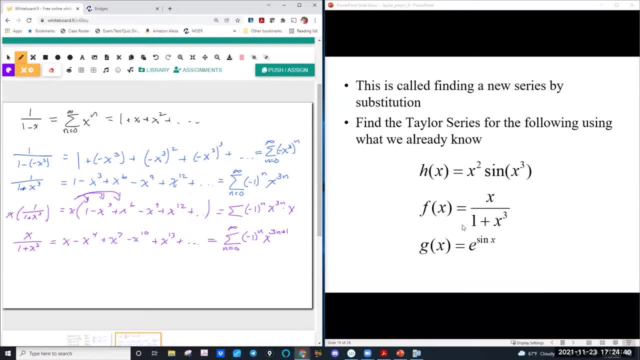 Okay, Questions about this. So we we found this Taylor series using a composition And also using multiplication. So those are a couple of methods of taking a known Taylor series And finding Using it to find a more complex Taylor series. Look at a couple other ways. 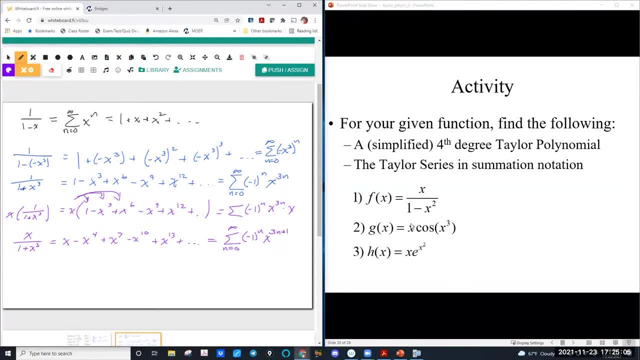 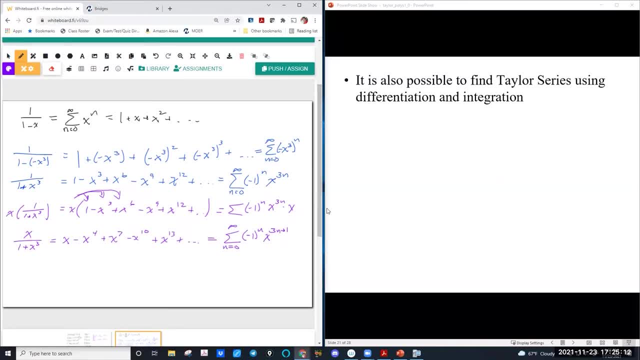 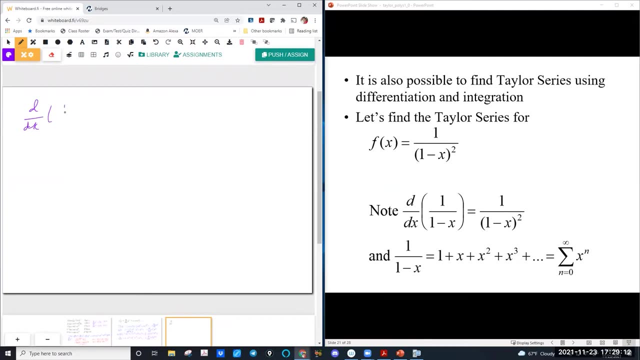 We're going to do that right now. We might come back to that To let you guys try some. We can also do this via integration or differentiation. So We know that the derivative Of one over one minus X Is one over one minus X. 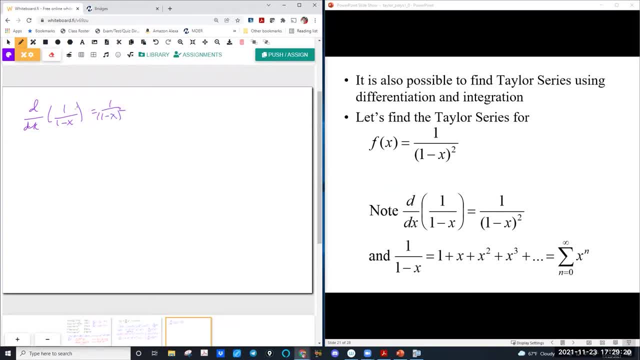 The quantity squared. So if we want to find it's Taylor series, we want to do the derivative Of the Taylor series for one over one minus X. So one plus X plus X squared, X cubed Plus, Very similar. We just take the derivative term by term. 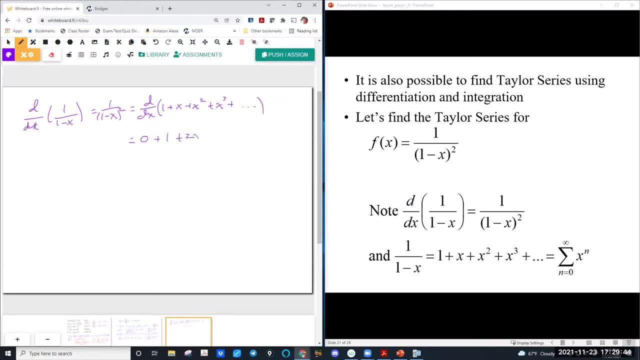 So we end up with zero plus one plus two X, Two X Plus three X. squared, That's only four X cubed Plus dot dot dot. And then for summation notation: Very similar Also. It was X to the end. 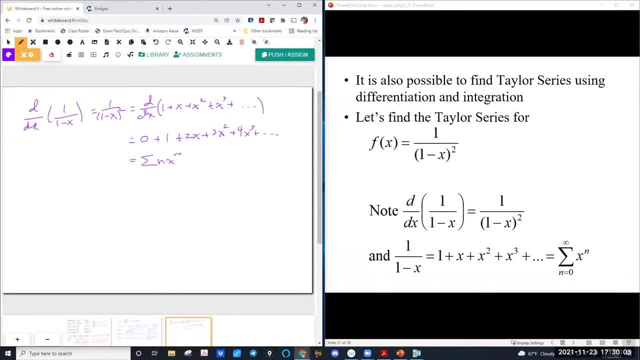 We take the derivative with our power rule and to the And times X to the end minus one. Now here, Because now We can actually Still- Yes, We can still- start this at zero, Because plugging in zero is zero. 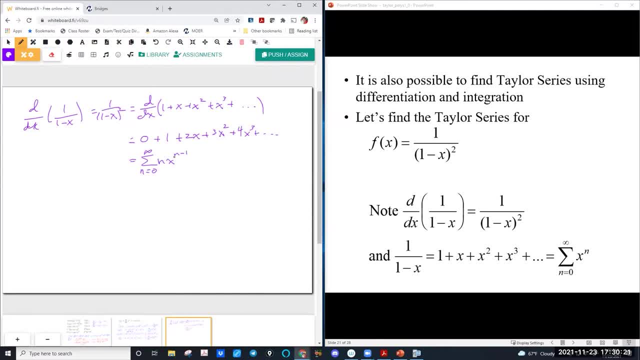 That works. Plugging in one, We give us one times X to the zero, which is one. Plugging in two gives us two times X to the first, So on and so forth. Now, I won't bore you with this one, but I. 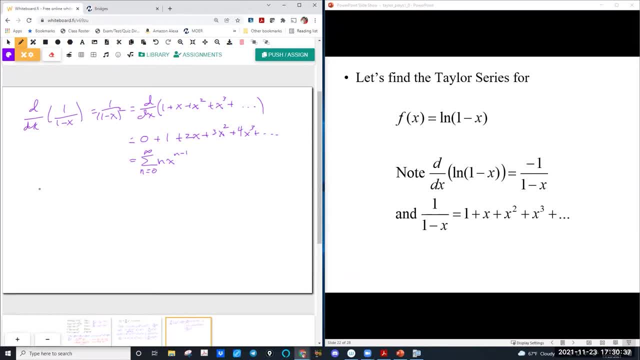 You know this one we're trying to do, Ellen- One minus X- And we know that the derivative of LN of one minus X Is negative, one over one minus X. So this is the one where we need the anti-derivative. 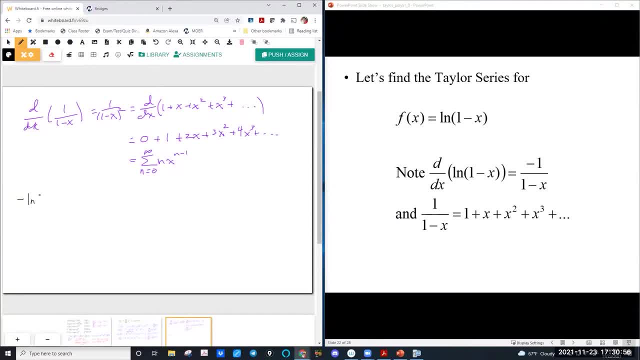 So here's what we know: Negative. I'm going to grade it this way: LN of one minus X Is equal to the anti-derivative of one over one minus X DX, And this is one plus X plus X squared plus. 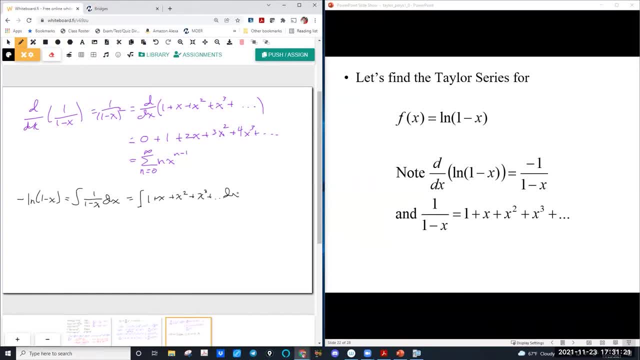 X cubed plus dot dot dot The X, And this is going to look really similar to what we did before. So we're going to have X plus X squared over two Plus X cubed over three. Dot dot dot. 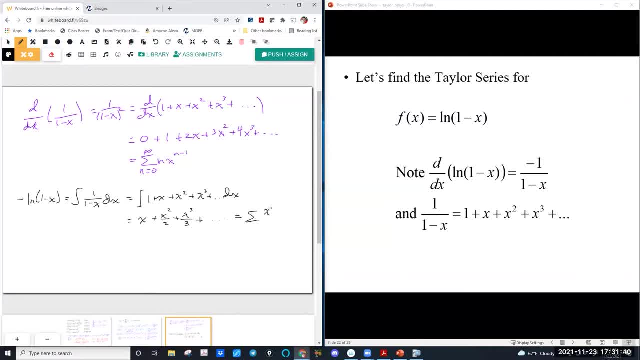 And that, As we saw before, Give us X to the N plus one over N Plus one From N equals zero to infinity. None of that has changed. Here's what's going to be a little bit different. This was, this is the Taylor expansion for negative. 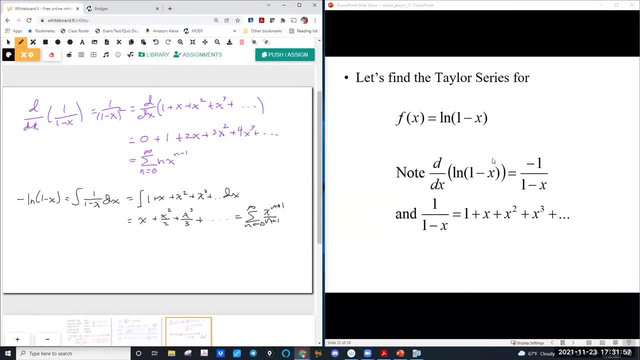 Ellen, of one minus X, This negative sign here. So If we want it for positive, So if we want the Taylor expansion for LN of one minus X, We have to multiply all the terms by a negative. So minus X, Minus X, squared over two. 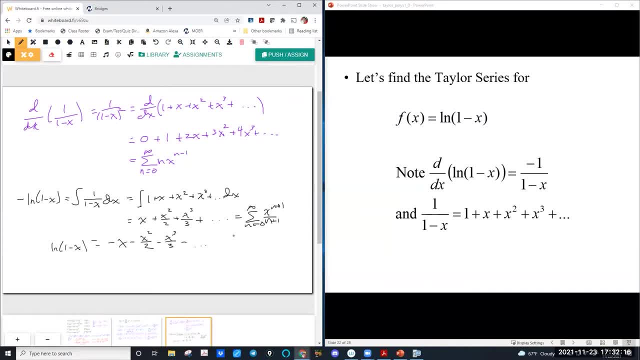 Minus X cubed over three. minus dot, dot, dot. And then we need to put a negative on our submission, And I'm just going to throw it out front. I think that's as easy as any place: X to the N, plus one over. 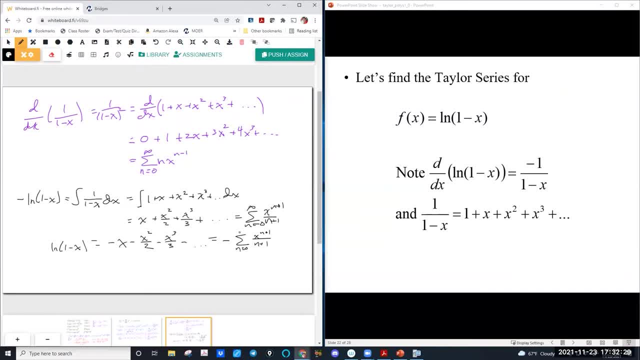 N plus one, And let it stay the same. I wanted you to see what this is, how we can use derivatives or anti derivatives To use a known Taylor series to find another one, And these methods can be combined. You could use an anti derivative. 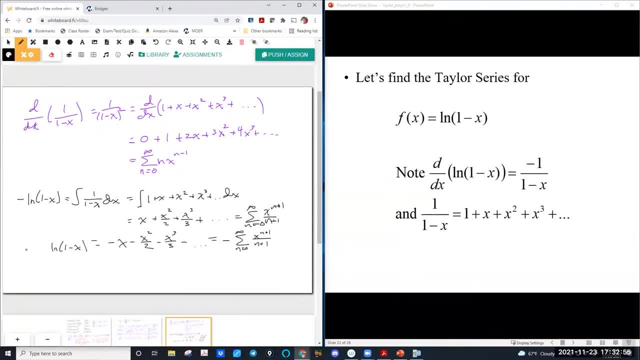 To find one. And then if you had to multiply by, Like, if we wanted to find, Say, you know just Just that, if we wanted to find X cubed LN of one minus X, We would take what we found here and multiply it by X cubed. 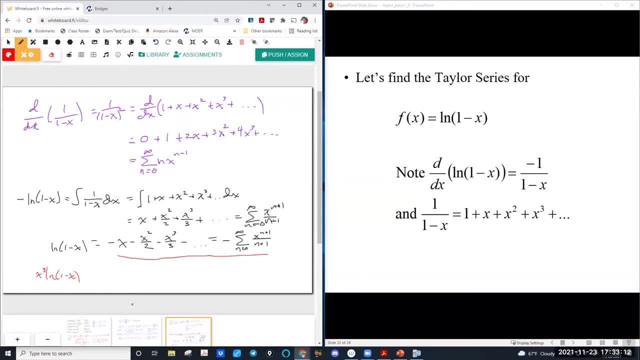 So all these methods can be combined. And What are the reason? I, like I want to show you all of these. It's not because we're going to do a ton of them, We'll do a few, and it's really usually pretty obvious. 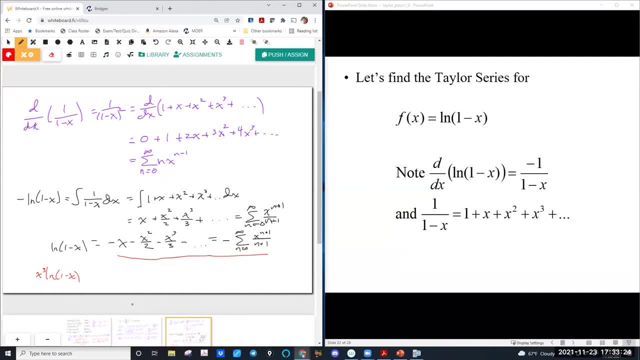 We're going to do a ton of them, But what you want to look for is if the derivatives look like they're going to get really messy really quick. What you want to look for is: Hey, is this a multiple or a composition? 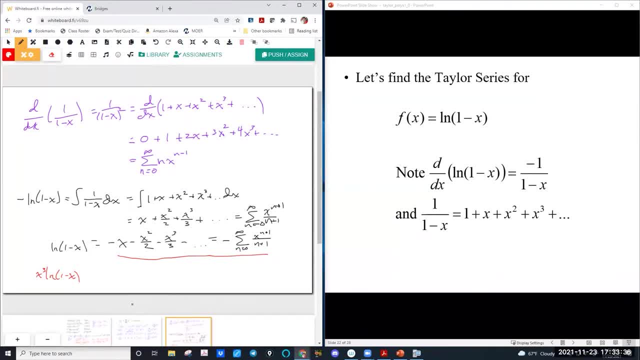 Or a derivative or an anti-derivative of one of our basic Basic ones. You know, is it a big cosine of X is a basic one. sign of X, Basic one. Either the X is a basic one, One over one minus X is a basic one. 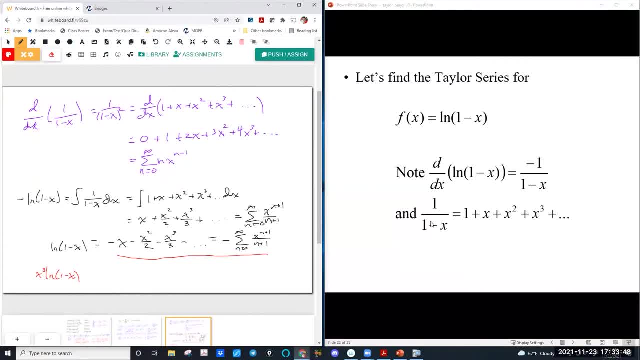 There's some basic Taylor Polo Expansions. Now We're going to look at some of these, The ones that we find and use often, And those ones are the ones that we look to use to see if we can find Taylor expenses for some of these more complicated ones. 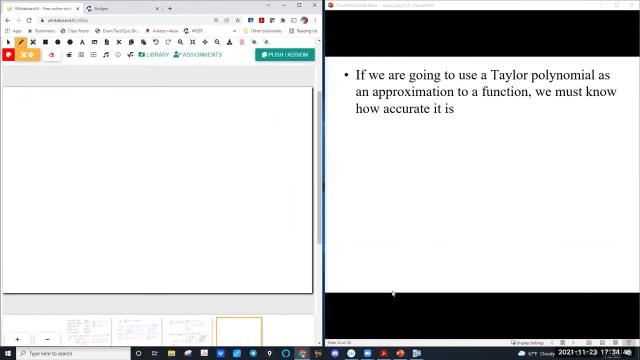 You know, because Taylor series and Taylor polynomials are an approximation, We always want to know how accurate they are. So, just like we did, Just like we had with our numerical integration, We have an error estimation. This is going to look really familiar. 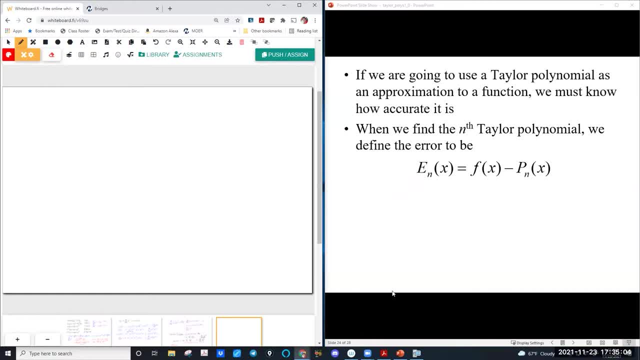 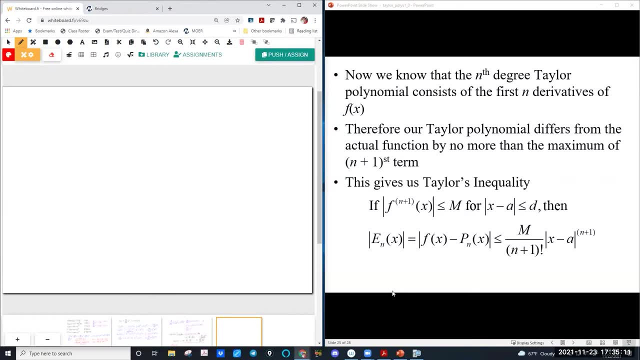 So Our error estimation for Taylor polynomials For the first nth degree Is given by what's called Taylor's inequality. This will look really familiar. This is you. This is what is used to derive those error formulas that we use For the midpoint rule and Simpson's rule and in trapezoid rule. 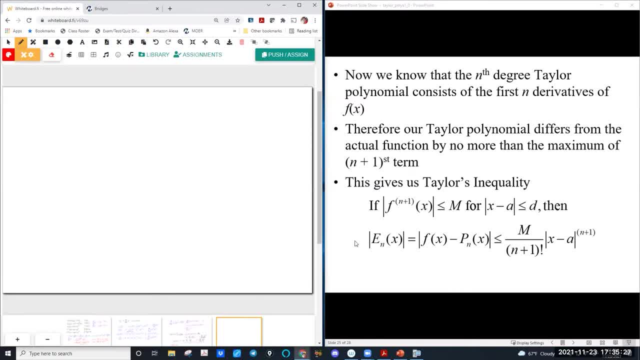 Back in our our numerical integration section. This is. this is exactly where it comes from. So you're actually doing a lot of the same stuff. So what I want to work on is how we use this in practice. Okay, So, 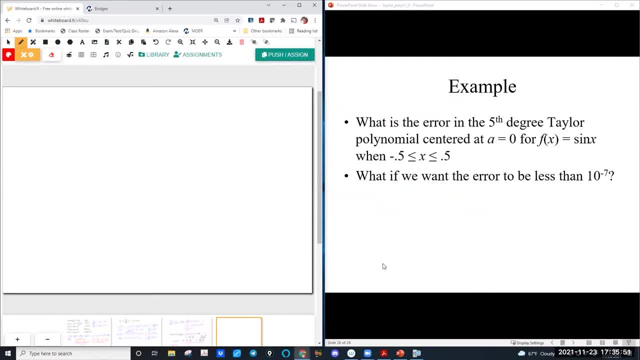 Let's go ahead and take a look at this one. This one's not too bad, But again it'll get us just kind of used to the air. So if we wanted the air in the fifth degree Taylor polynomial centered at equals zero, 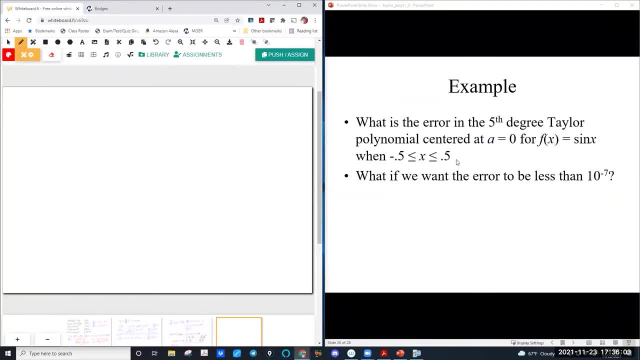 For F of X equals sine X When X is in between negative 0.5 and 0.5.. We can use that approximation. So We want a fifth degree For sine X. We don't have to for this one. 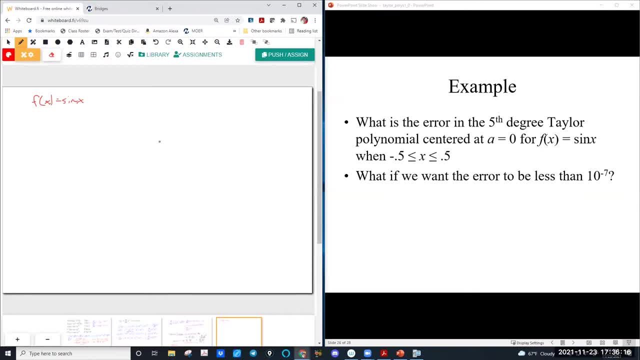 we don't actually have to find it. We certainly could, Because we know that. We know that this is one of our basic Taylor series is centered about zero, But We don't need it. So here's here's the way that this works. 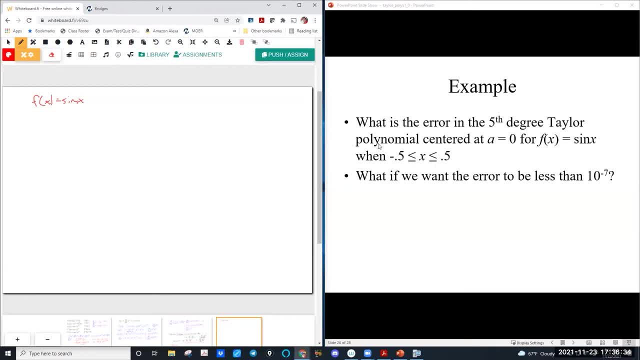 So we know that we're in between negative 0.5 and 0.5.. We're in the fifth degree And I want to bring the air back up. That's one right. This stuff down With the fifth Degree. 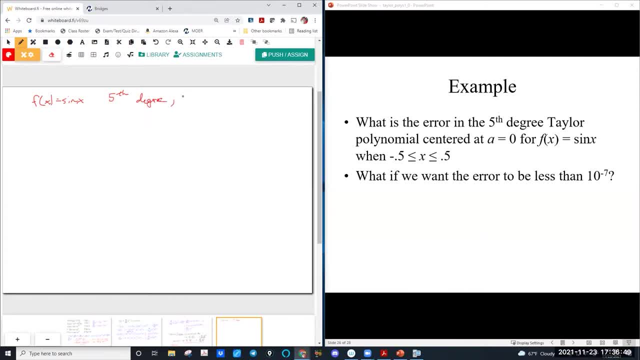 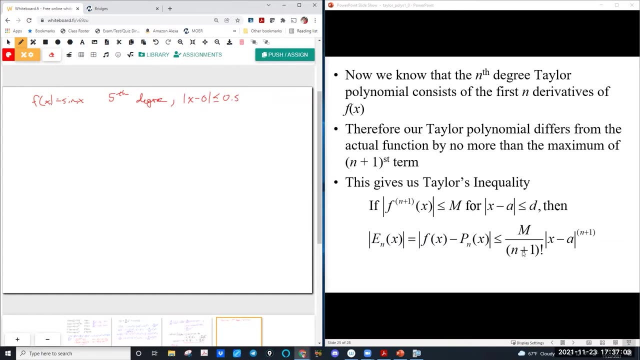 Taylor polynomial, And we know that the absolute is centered at zero- Is less than or equal to 0.5.. Okay, So we see a lot of this stuff is going to pull right out of there. So if I go back to our, our term, 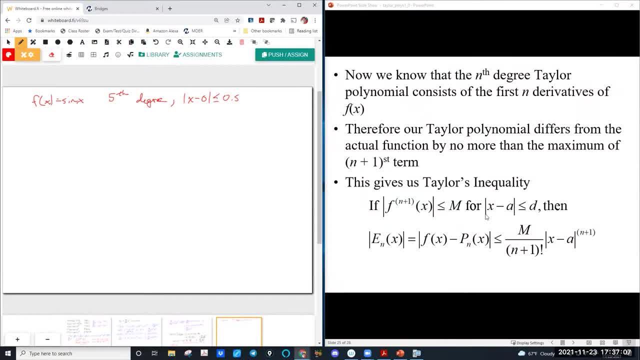 It's M Over M plus one. factorial times X minus eight to the N plus one, As long as X minus a is less than D. Okay, So the D Is this 0.5.. This here Is our D And you'll see and I'll show you why that's important. 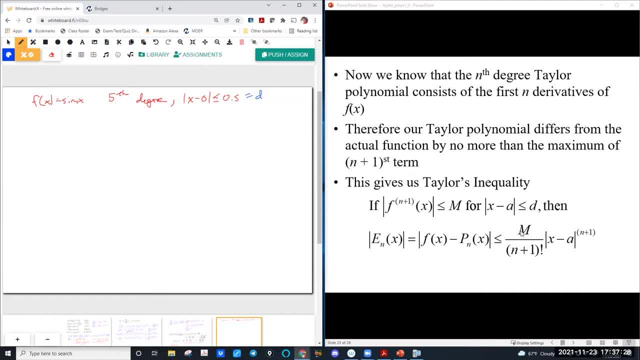 Um, Now here's what we need. We need This is where all the work is done, just like it was Back in those take home problems for the midterm. Well, the thing about sign is it's derivatives are all either sign or 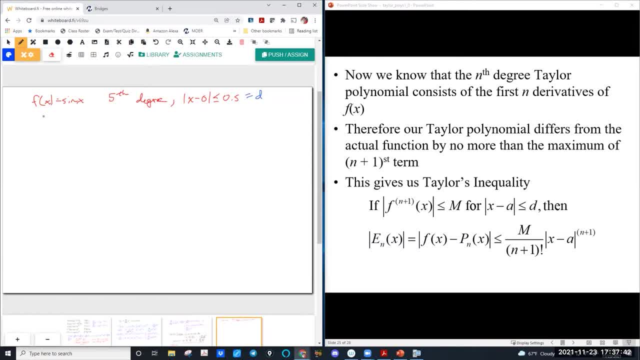 Our sign or cosine plus positive or negative. So we know That the uh we have to bound the sixth degree Derivative Derivative. We know that the sixth derivative It's always going to be less than or equal to zero. 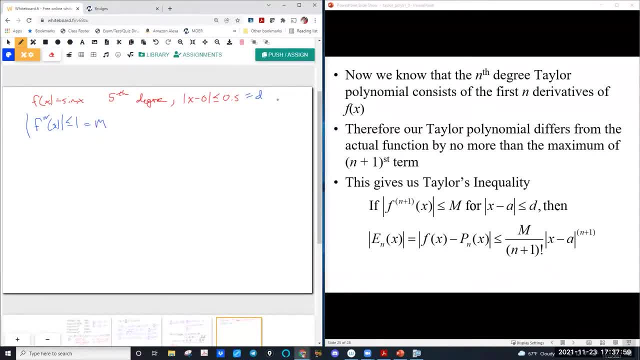 Or equal to one, So we're going to use that for our M. So here's how this works, And it's a fifth degree, Sorry, And his five, Just to get you used to how all these pieces work. So we know that our error. 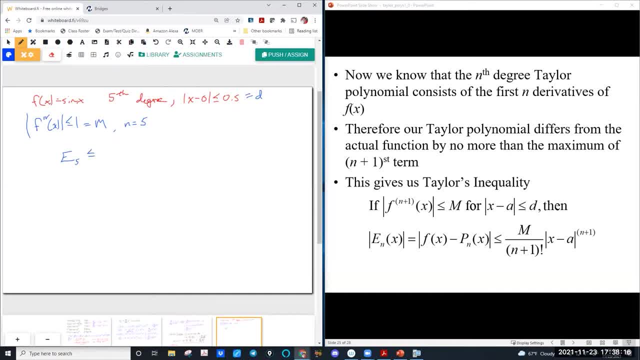 In the fifth degree Taylor polynomial It's going to be less than or equal to One over Six. factorial That's the N plus one Times The absolute value Of X To the sixth. So the question is okay. well, what about this part? 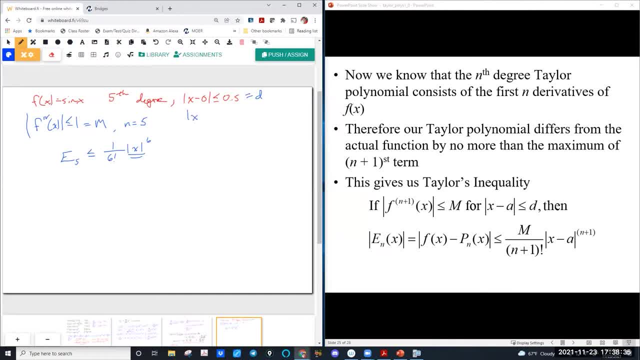 That's where this comes in. This is saying The absolute value of X is less than or equal to 0.5.. So what we're going to do is replace. the absolute value of X was 0.5. So we get one over. 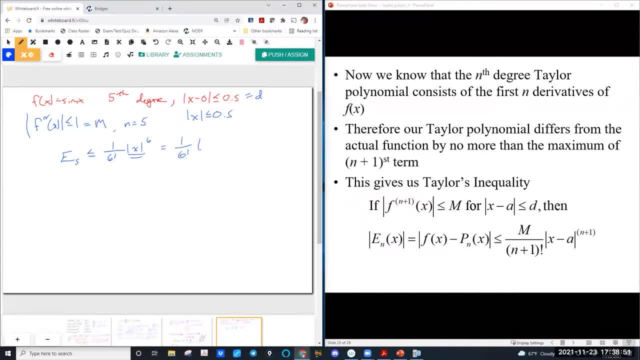 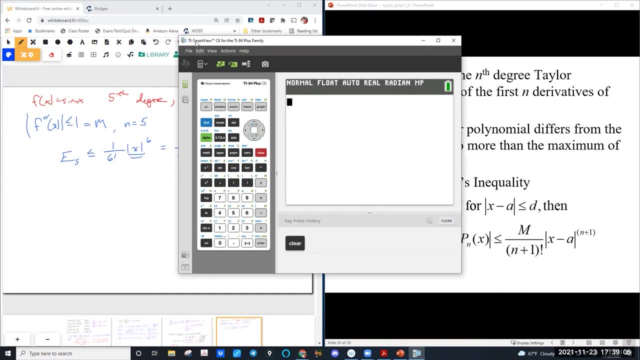 Six factorial Times, 0.5. To the sixth. That is going to give us our error estimation. So if we want to, that's something we. if we want that, you know we might need the number. We might want to do a comparison. 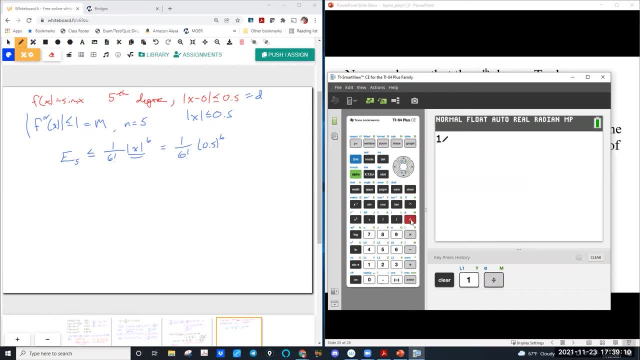 This is something we can do in the calculator, So if you're not sure where the factorial is, Let's go through that. Now You're under math, It's going to be under probability, and there's your X Exclamation point. 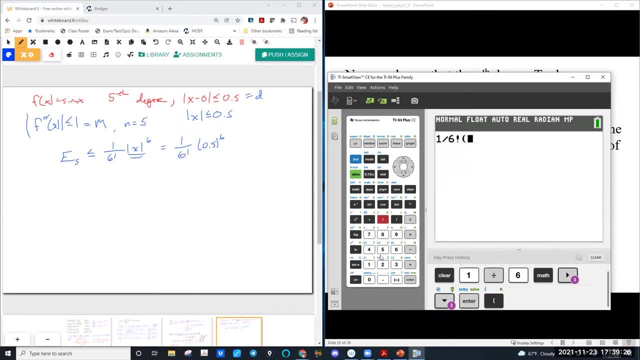 So there's our one over six factorial, And then times 0.5. Raised to the sixth, So a really small number, And it's Because we have such a high degree polynomial and such a small interval. So this is what: 2.17 times. 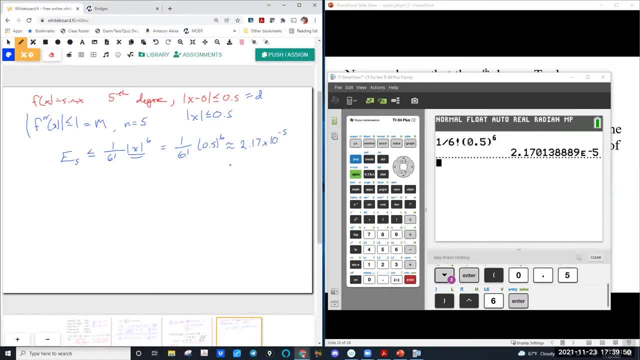 10 to the negative fifth, Or You know, if we wanted to write it, It's going to be Not in scientific notation: 0.2.. One, Excuse me, End of zeros: 0.000.. 2, 1, 7.. 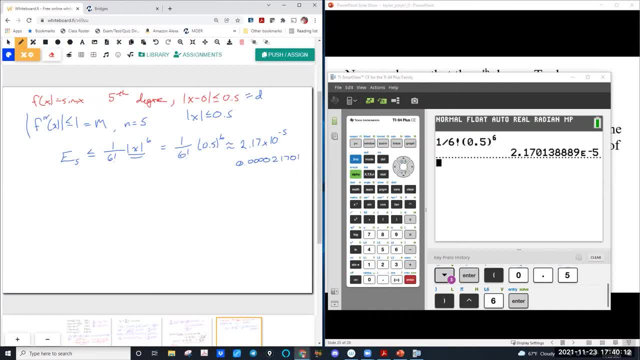 And then they however many digits we need For our problem. So it's going to be a really small error And it's because we're on such a small interval. So We have the The Power of Polynomial Taylor. 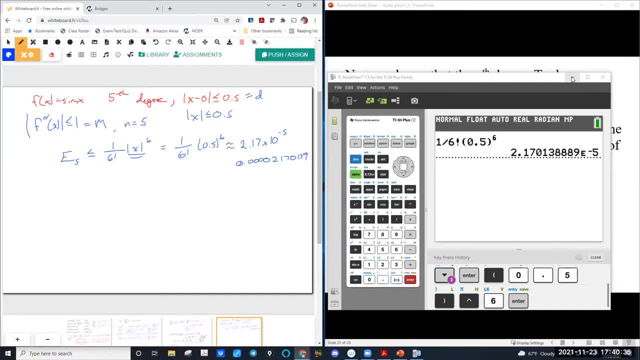 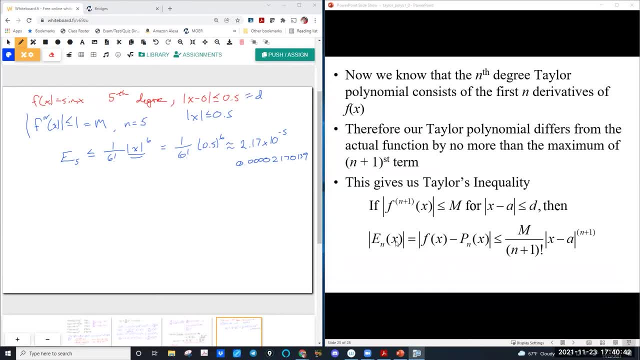 Again, guys, you have dealt with this error estimation stuff before And it's very similar. There's only a couple of small differences, But Question is so far. So the N is the degree That we need to calculate, What we need to calculate? 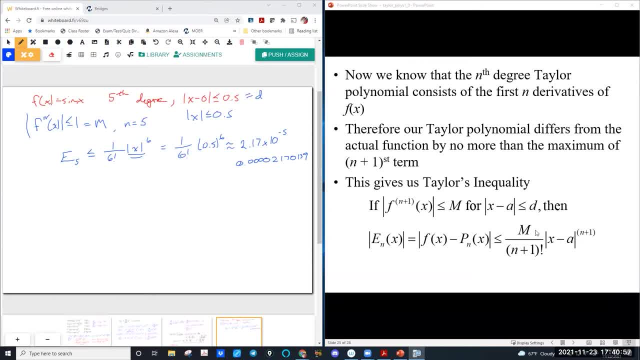 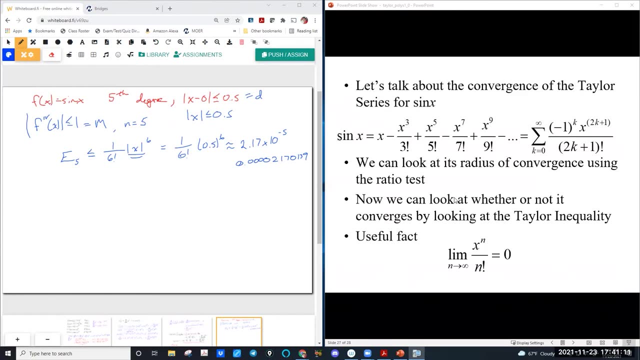 X minus a is basically going to be given in our problem. We're going to do another example here in a sec, But I want to see if there were questions about this one. Okay, So We'll come back to this, but 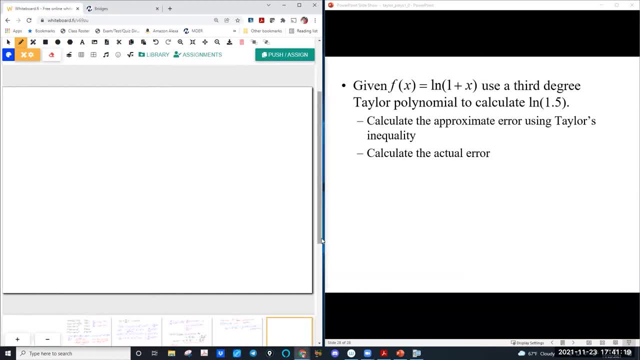 Here's what I want to look at: is this, This is going to be? This is this is going to be Some of the stuff we did earlier, Some of the stuff we did on Thursday, Some of the stuff we did earlier today. 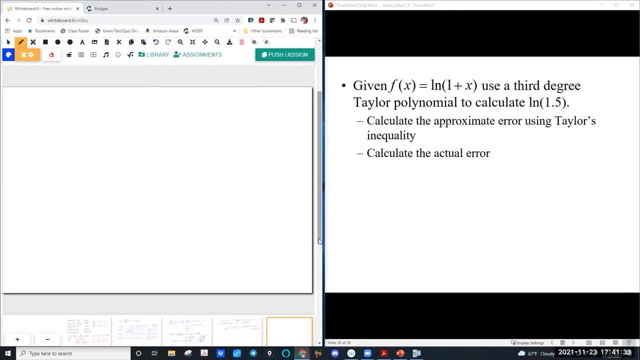 And this is going to be What you need to know for the first take home problem. for the final, which is as we talked about last time, is now available. All right, Let's see what we're asked to do. Half of X. 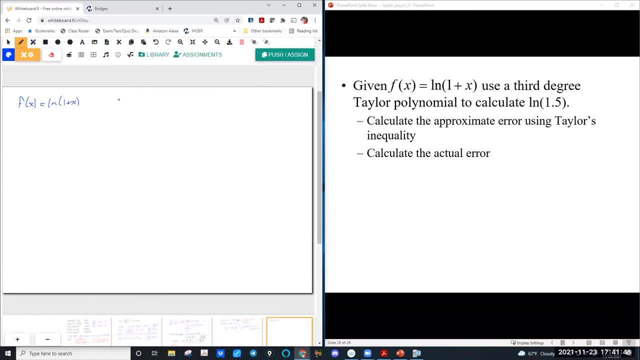 Is Ellen, One plus X Is Ln, And we want to approximate Ln of 1.5.. Now, Ln of 1.5 can be done in any calculator, So we know the exact value. What we want to do is figure out what the maximum possible error is. 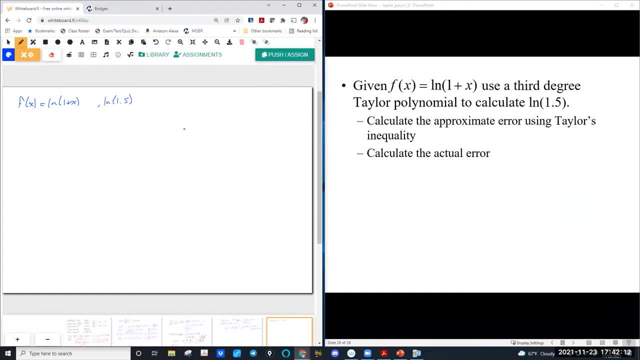 Calculate the actual error and see how far off we are using a third degree Taylor polynomial, Which means we're going to need at least the third. We're going to need up to the third derivative. I don't think I have this set up in just a sec. 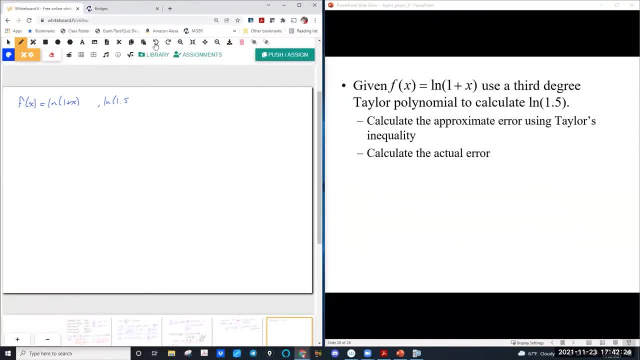 Let's put that off to the side. Our goal is to approximate Ln of 1.5.. Okay, So, first off, Something we've done before: the third degree Taylor polynomial- That we should be getting better at at this point. So 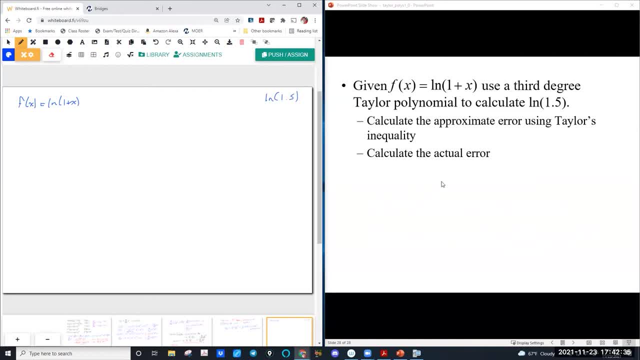 F of Ln. Ln of 1.5.. Okay, So, first off, Something we've done before: The third degree Taylor polynomial That we should be getting better at at this point. So F of 0.. Ln of 1 is 0.. 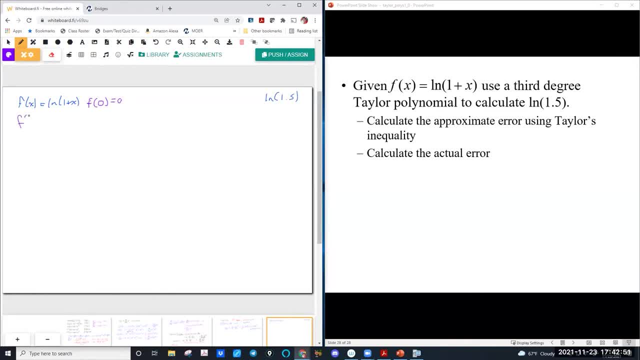 F of 0 is 0. So now we start finding derivatives. F prime is 1 over 1 plus x, And this may be easier to do Written as 1 plus x To the minus 1.. All right, Because that right there, we know that our F prime of 0 is just 1.. 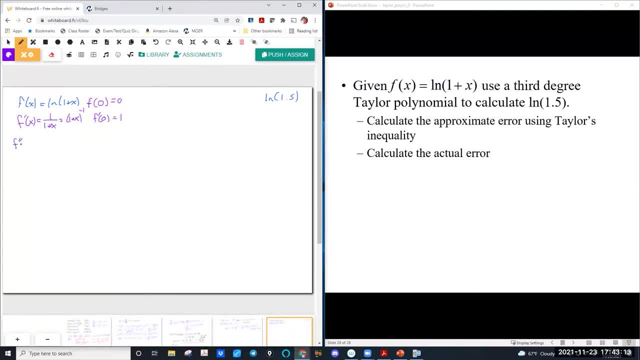 Because 1 to the negative 1 is 1.. But this is going to make it easier to find our derivative. So F double prime Is negative 1 plus x to the negative 2. And F double prime of 0.. 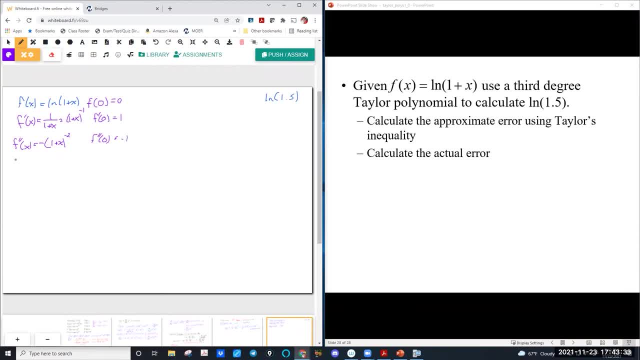 Then is negative 1. We can already probably start to see. Okay, It looks like we might have an alternating series here, But let's check it out. F: triple prime of x- We're going to need this one for the third degree, Taylor. 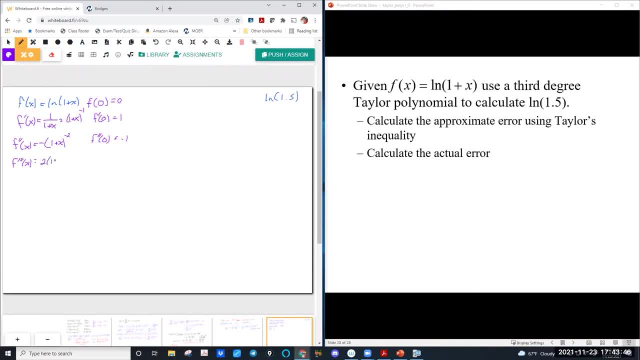 Negative 2 times negative. 1 is a positive 2. 1 plus x to the negative 3. F triple prime of 0. Is going to be 2.. And we are going to go one more Because we're going to need it for the error term. 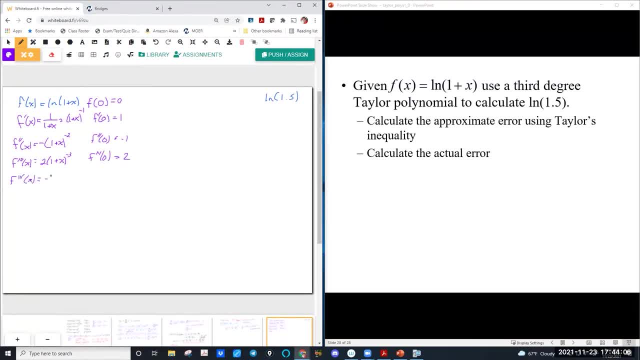 Because we need the n plus first. Well, that gives us negative 6 times 1 plus x to the negative 4th And F. The fourth derivative at 0 is negative 6.. We now have enough to build our third degree Taylor polynomial. 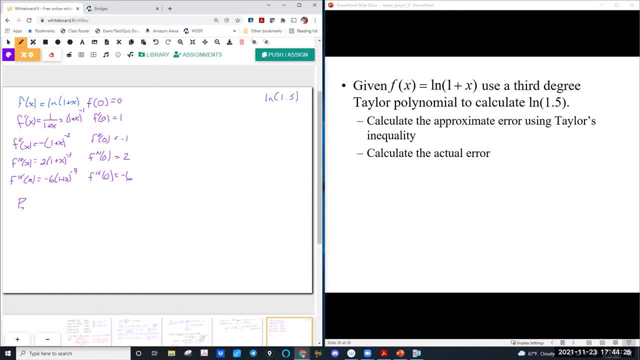 So our third degree. This is exactly what we were doing before. I'm going to write it out and then we'll simplify it. So 0. We're centered it. We're going to center this at 0.. It didn't say in the problem. 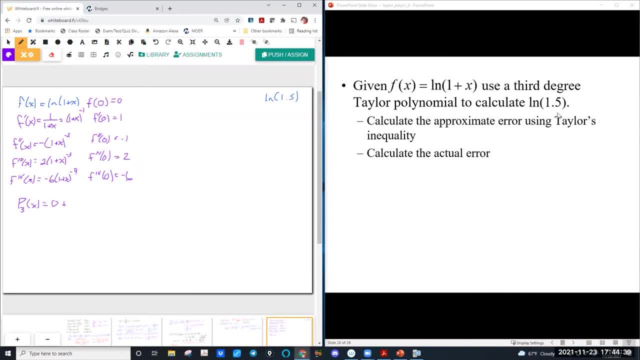 But we're going to want to center it at 0.. Because we're just estimating it all in a 1.5.. So we're centered at 0.. So 1 times x to the first Minus 1.. 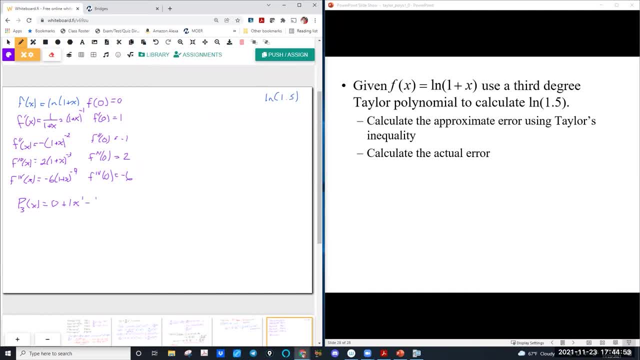 Over 2 factorial X to the second, Plus 2 over 3 factorial X to the third. We're done. That's a third degree Taylor polynomial. Remember this extra term Was for when we go to linear The error. 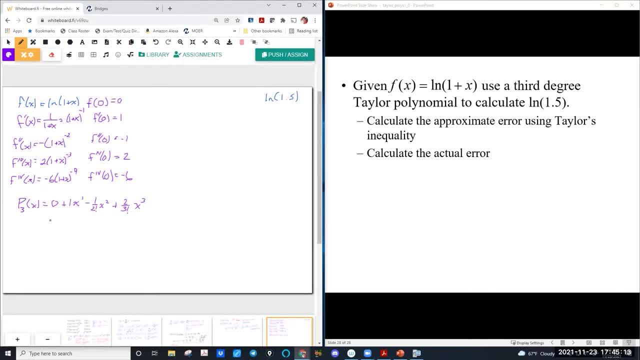 So let's clean this up a little bit. We don't need the zero, We don't need the ones, So we have x. 2 factorial is 2.. So minus x squared Over 2. 3, factorial is 6.. 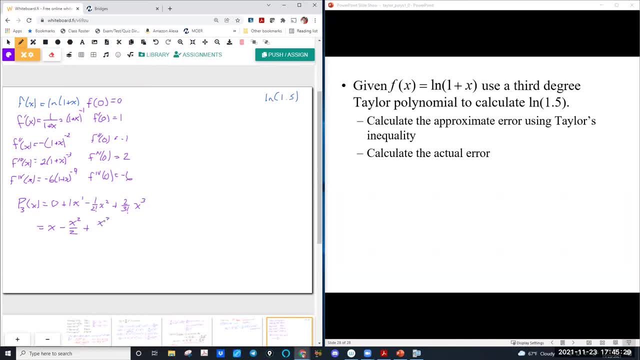 But 2 over 6 is 1. third, And I probably don't even need to go any further. You probably, If we needed more terms, I bet you could figure out the pattern on this one. But we were asked for a third degree Taylor polynomial. 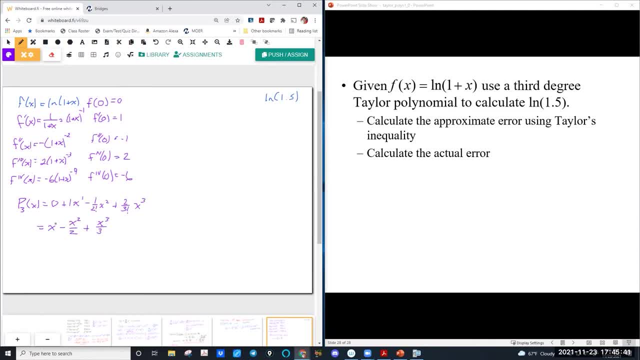 And that's what we got. Okay, So there's the third degree Taylor polynomial. Now Let's talk about calculating The error. Now here's where Here's. this is pretty interesting. So our function is ln of 1 plus x. 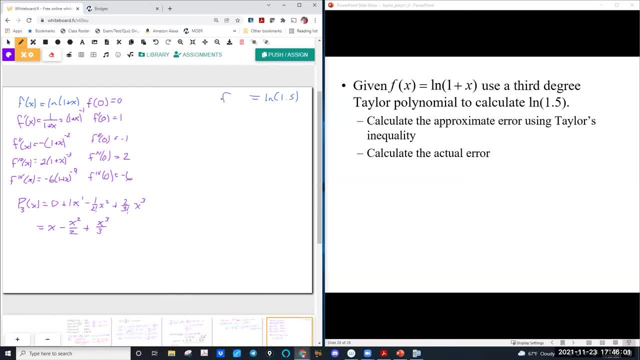 So ln of 1.5. Is actually our function Evaluated at 0.5.. Okay, Because If I put 1.5 in, We'll give us that. So that's one of the things you got to be careful of. 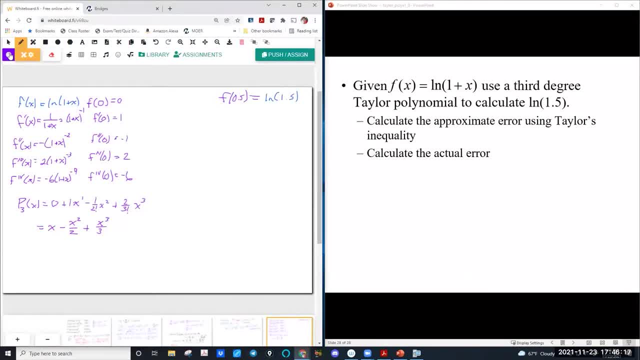 I don't want to put 1.5 in here, Because then I'm calculating 1.5.. So when I, When I go to find my approximation, I'm basically going to be putting in 0.5. Into my. 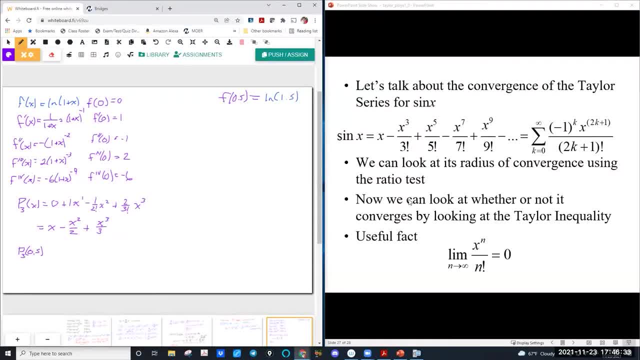 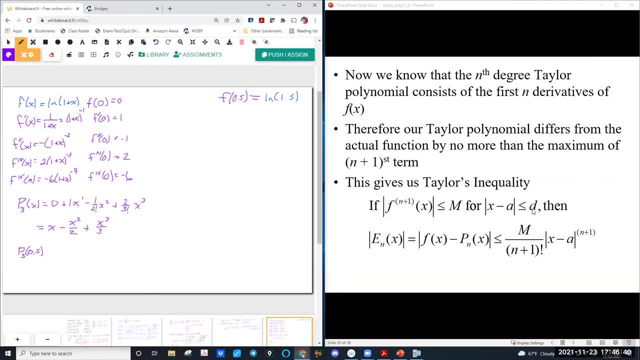 Taylor polynomial. Now here's why that's important. Let's go back to our error term, So you guys can see it Here: X minus a has to be less than or equal to d, So Our d Is going to be 0.5.. 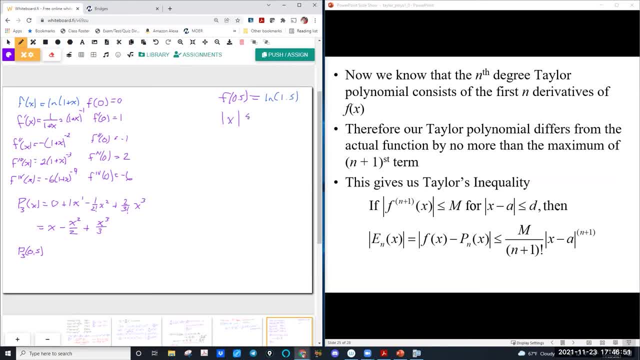 So we get the absolute value of X Less than or equal to 0.5.. Now The last thing we have to do Is Find the. We have to maximize the n plus first derivative On this interval. So 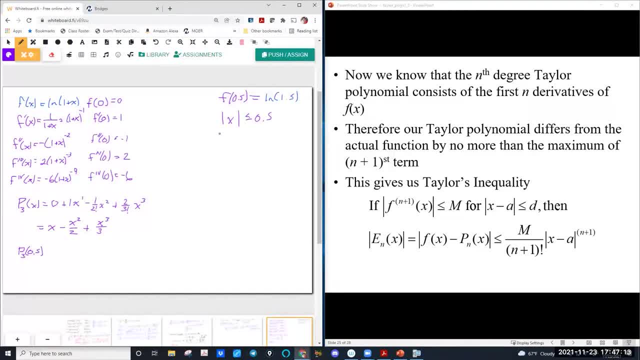 If the value of x is less than or equal to 0.5.. We're actually on the interval From Negative 0.5.. Up to 0.5.. Now We'll also look at 0 on this one. 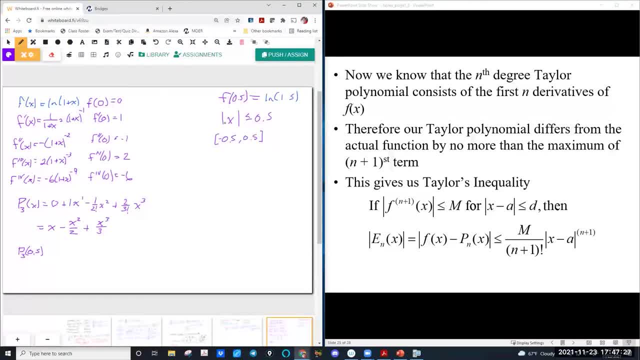 Because something interesting is going to happen there. But I want to do it On the full interval first, And then we'll look on the half interval. So I want to show you something. Okay Now. So We're minimizing a function. 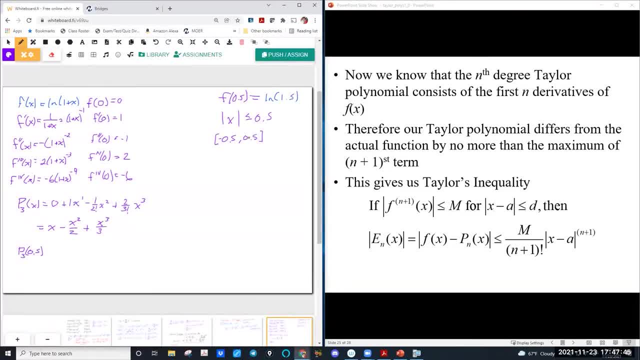 It's on a closed bounded interval which we're on- Happens at one of two places, either at an end point Or at a critical point. We can take the fifth derivative, but our only critical point Is going to be at negative one. 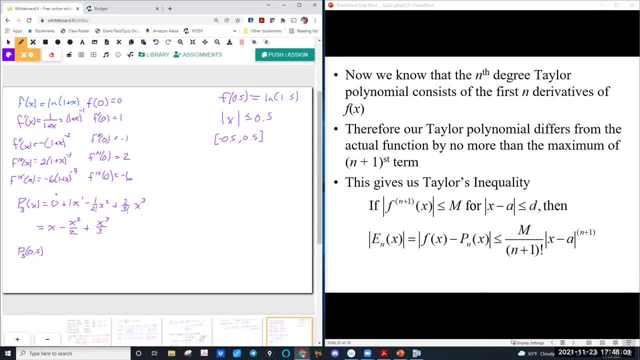 because that's the only thing that makes this Actually discontinuous. Doesn't even make the derivative zero Negative. one's not in our interval, So we're going to take the fifth derivative At negative 0.5.. Which comes out to be: 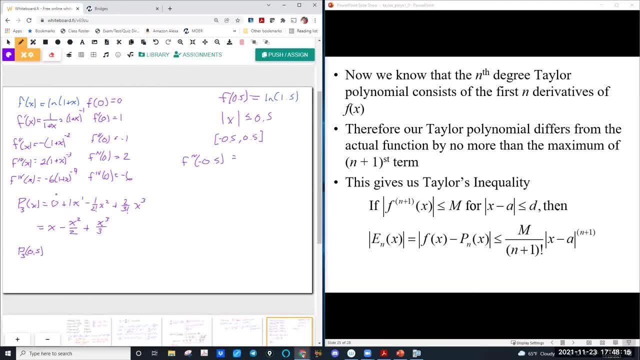 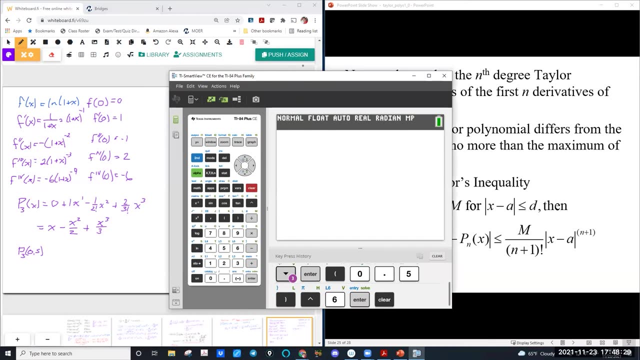 I believe 90.. Let's see, I can't read my own handwriting, So So remember what we're doing. We're plugging this into the fourth derivative, So we have Negative six. Actually, we don't care about the fourth derivative. 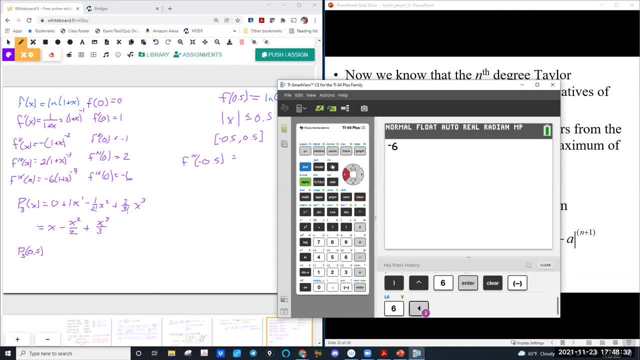 We're plugging this into the fourth derivative Here And we're going to do positive or negative. So, Because we want the absolute, the biggest magnitude, One minus 0.5.. Raised to the negative: 96.. Okay. 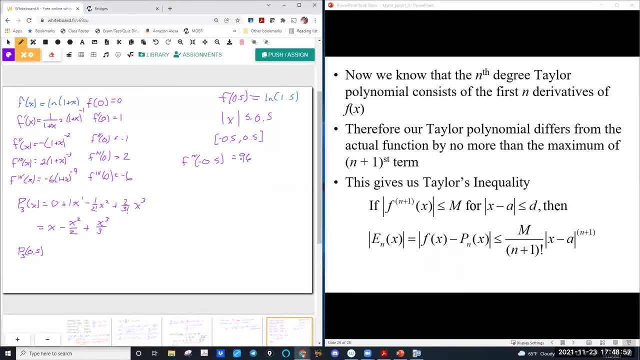 I couldn't tell if I wrote 90 or 96. So I wanted to check, So that's 96.. All right, We'll also do our derivative At 0.5.. Same thing: You plug in 0.5 into here And for this you get as a fraction, you get 32 over 27.. 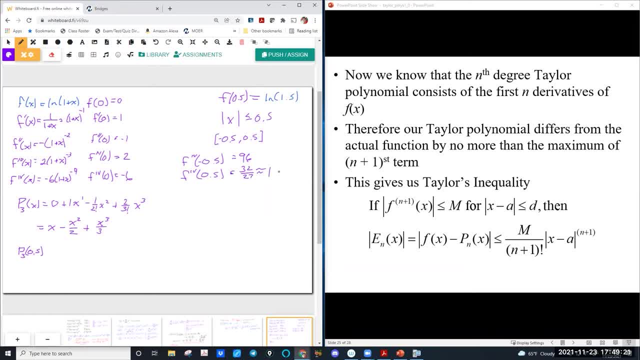 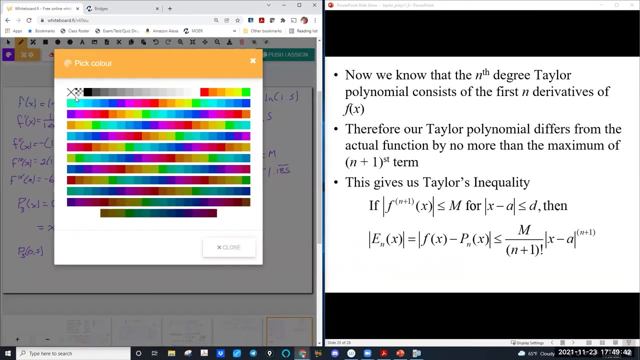 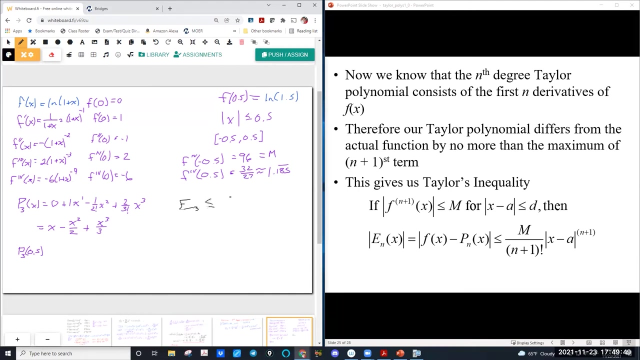 If you want it as a decimal, it's 1.185.. And those terms are going to repeat. Okay, so clearly this is going to be our M. So our error estimation for the third-degree Taylor polynomial. we know that the error in our third-degree Taylor polynomial is going to be less than or equal to our M, which is going to be 96 over 4 factorial. 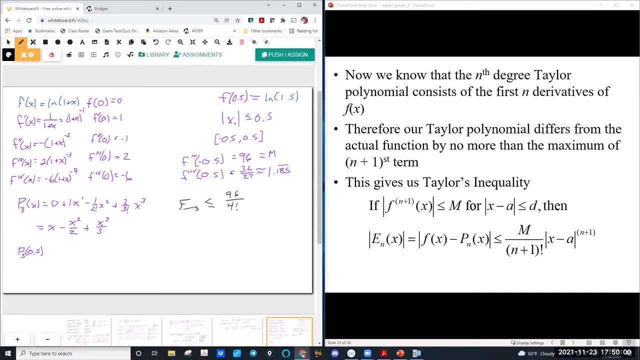 Now the X minus A. well, X minus 0, it's going to be the 0.5.. And then to the 4. These numbers are always going to match. If you calculate that, we actually get a pretty big number on this one because of the negative 0.5, which is 0.234375.. Pretty big. 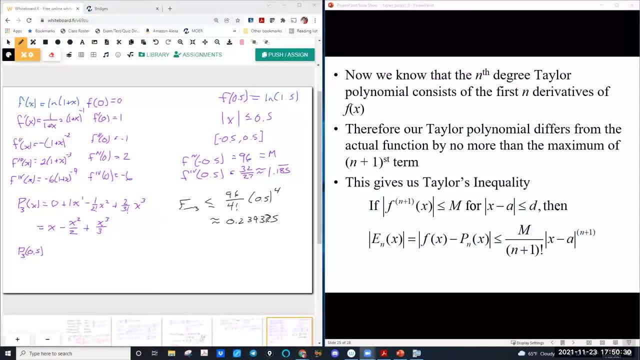 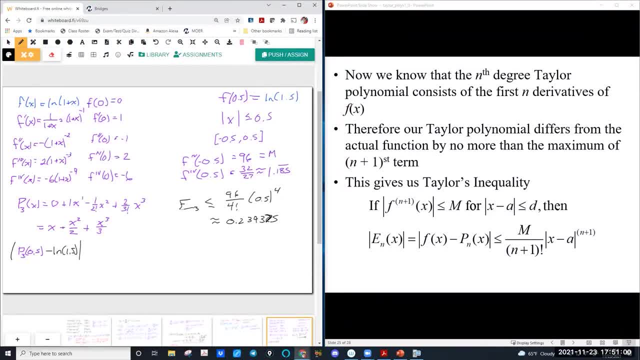 So we're going to subtract off the absolute value of this. Now, the way this is computed, you're just putting 0.5 into x. here You can use a calculator or Wolfram or something to calculate that And we'll subtract off the ln of 1.5.. 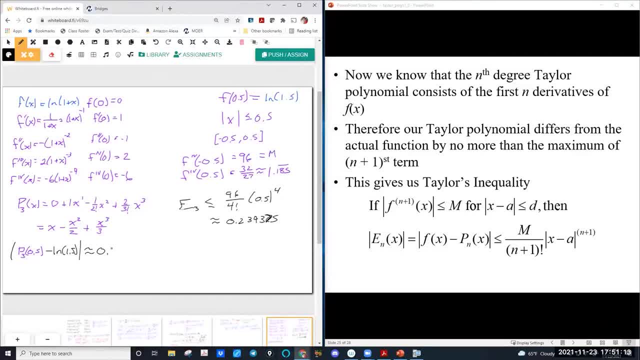 And we get a considerably smaller error than our estimate: 0.0112015586,, which is definitely less than 0.234375.. 0.03108641375.. OK, Again, it's a very conservative error estimate. Now, one of the things that ‑‑. oh, actually, before I go on, any questions about this one. 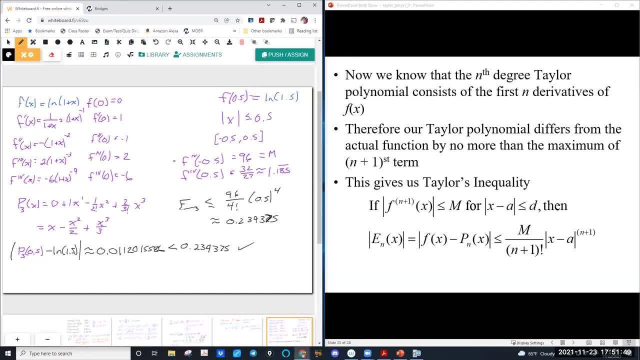 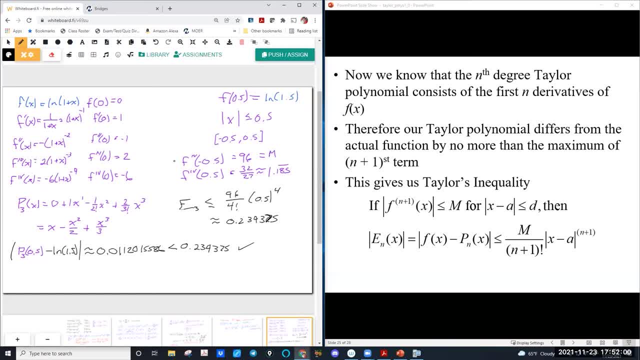 Right, It's almost again. the error formula is derived from this Taylor inequality, So you're really doing a very similar procedure. Now, one thing that I like to show on this one- and it happens on a lot of these, because this thing is centered at zero. we could have actually let's do some different colors to make it obvious that it's not part of this one. 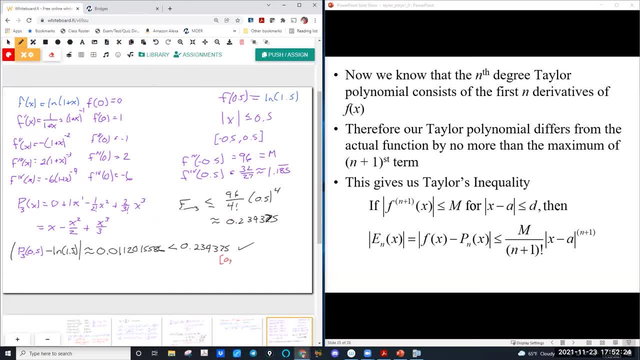 We could have done it on the interval from zero to 0.5.. This is a little bit less conservative but because of the type of function we have and we're all the way out at the end point, we could actually do it on this interval. 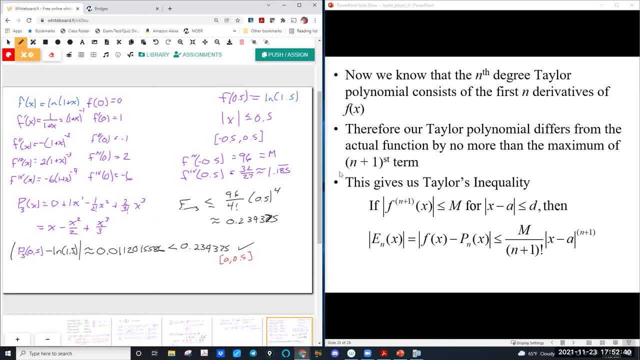 I want to show you guys both ways. This is the way off of the definition, but a lot of times we're only dealing with like half the function. You can go from where you're centered out to where you're interested at Now. the only change that this makes is, instead of checking this one, we do our 14..